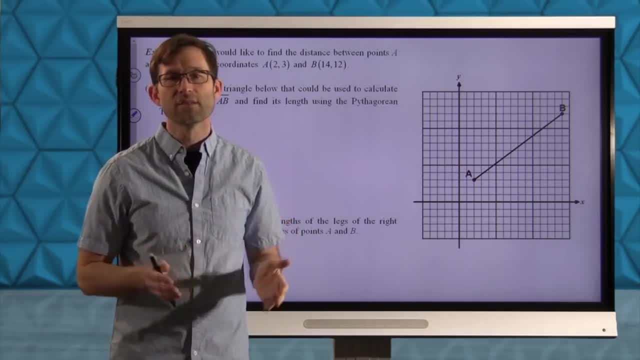 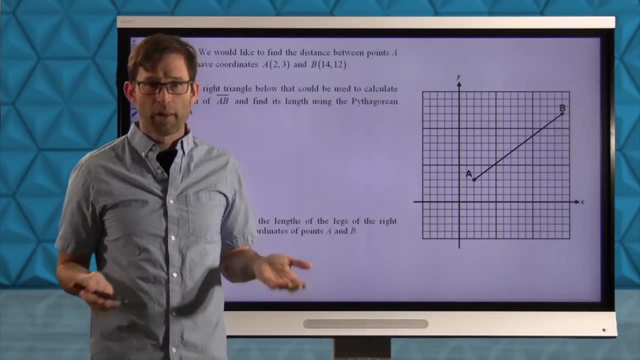 segment that connects those two points. So length and distance truly truly are the same thing. So that's the length formula, but we generally call it the distance formula. Alright, let's take a look at exercise number one. We would like to find the distance between points A. 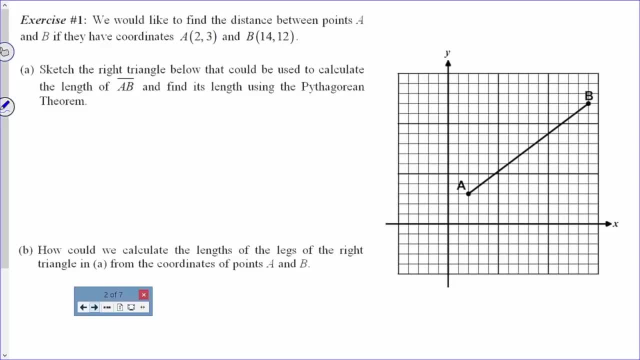 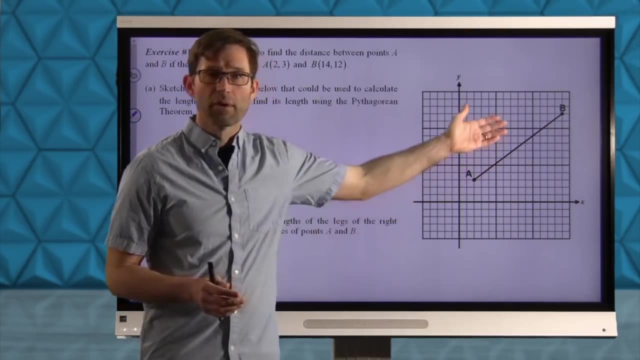 and B if they have coordinates at, and Letter A asks us to sketch the right triangle below that can be used to calculate the length of AB and find its length using the Pythagorean theorem. So one of the cool things is whenever you have a line segment in the coordinate plane. 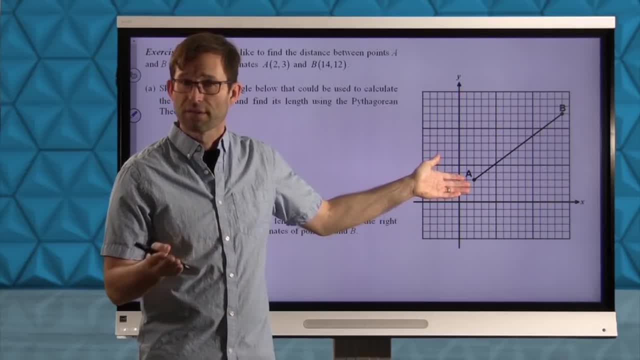 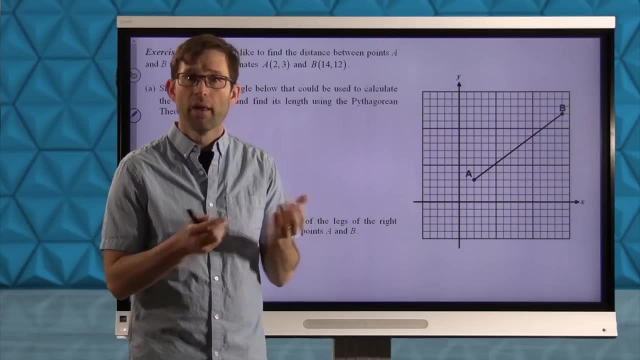 that's slanted. That's slanted. So it's not horizontal, it's not vertical, but it's slanted. Then you can always think about that as being the hypotenuse of a right triangle, And let's draw that right triangle. 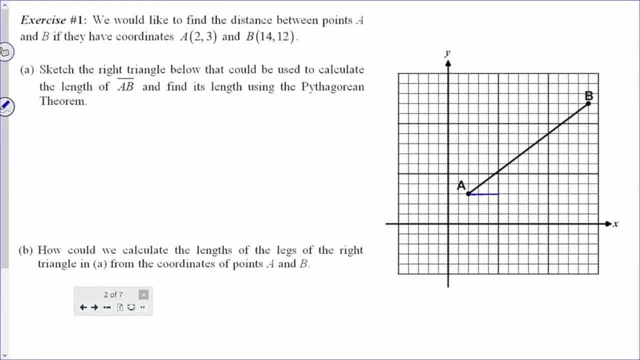 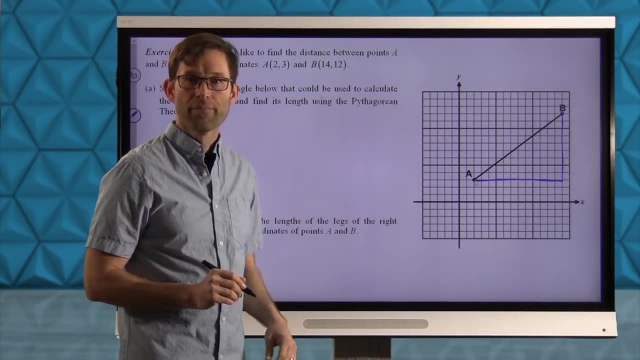 in together. Specifically, we can have this particular right triangle. Let's see if I can. Alright, And of course, you can note, while looking at that right triangle, that AB is its hypotenuse. In fact, let's draw it out right here. 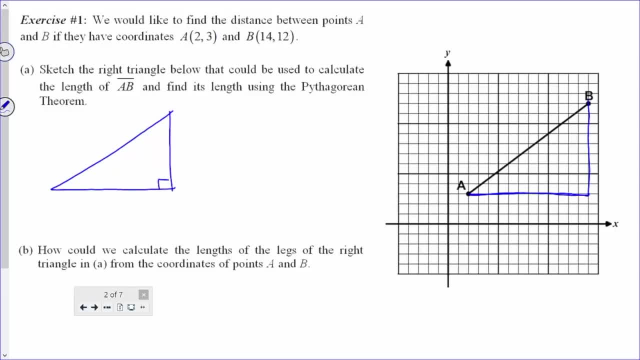 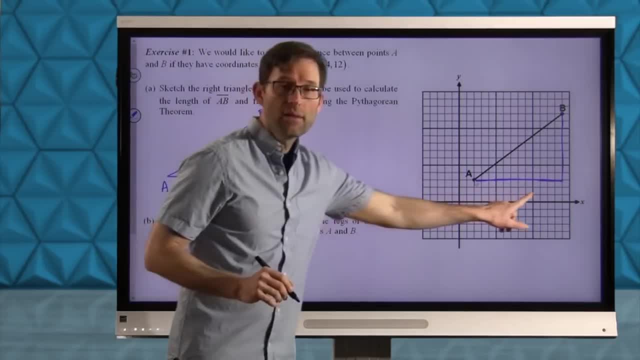 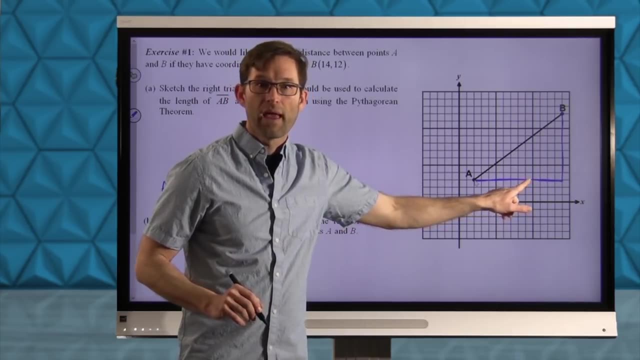 OK, Of course any vertical line is perpendicular to any horizontal line. Alright, That's what gives us that right triangle. And now I can literally just count to figure out how long this is. And what do I have? I have three units here, then I have another five units, so that'll be eight and another. 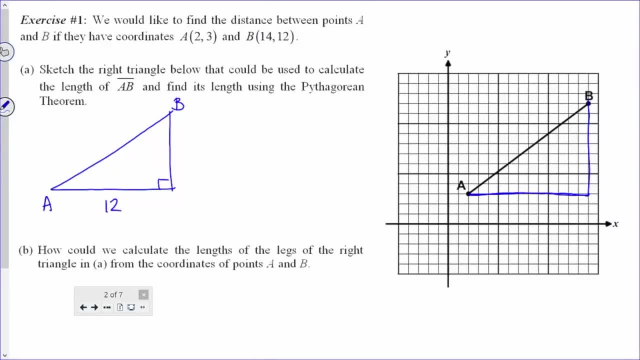 four units, and that'll be twelve. Likewise, I can also think about this vertical distance. What do I have? I've got three units and I have another five units, so that'll be eight and another four units, and that'll. 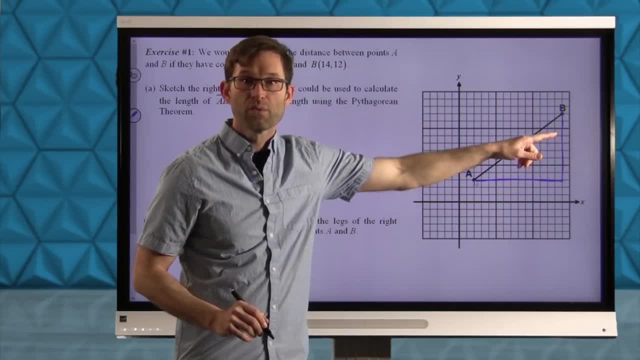 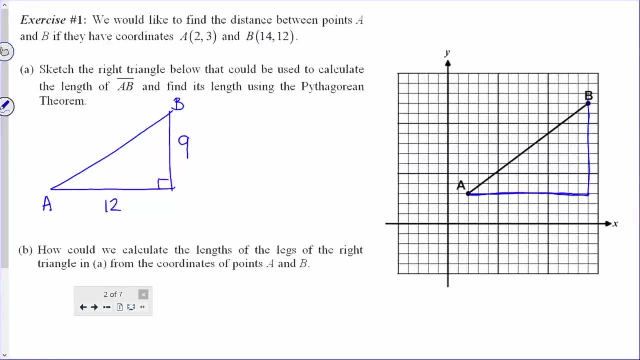 be twelve. Likewise, I can also think about this vertical distance. What do I have? I've got two units up to here, another five units, which is seven, and another two units, which is nine. Is that right? Yeah, Nine units here. 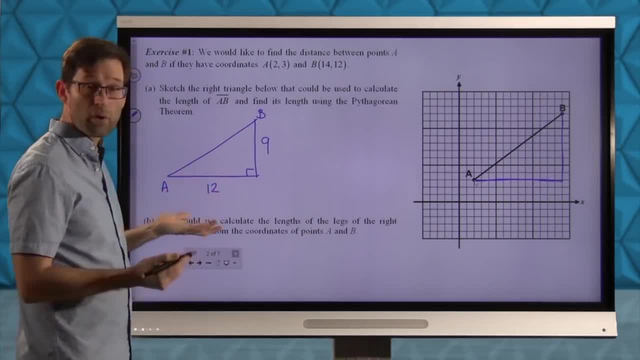 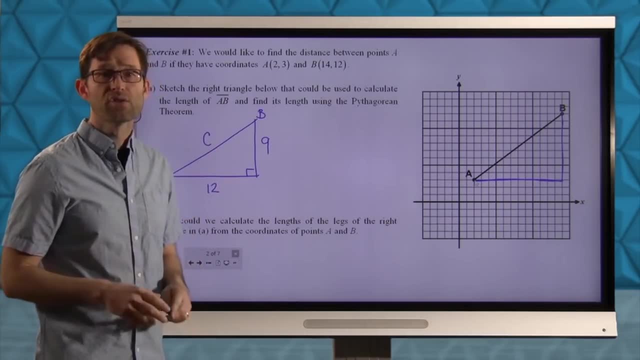 So therefore, the length of AB right- which is what I'm looking for- or the distance between A and B is the hypotenuse. So take a moment now and pause the video and solve for the length of the hypotenuse. 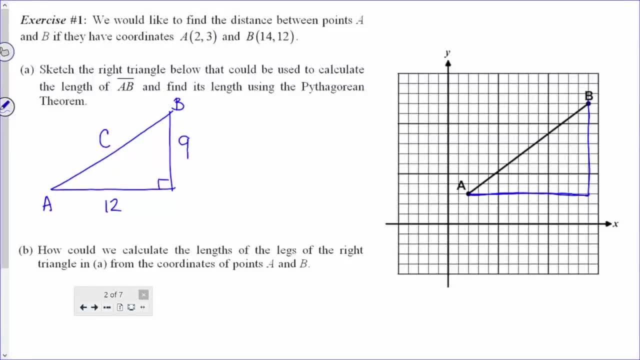 of that right triangle. Alright, Let's take a look at the right triangle. OK, Alright, Let's do it. So what do we have? We've got nine squared plus twelve squared is equal to C squared. Nine squared is eighty-one. Twelve squared is a hundred and forty-four. You can always. 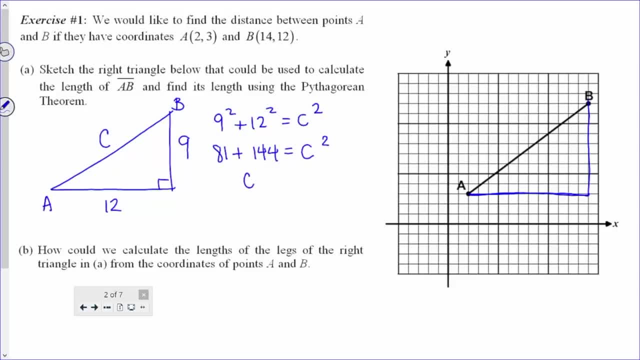 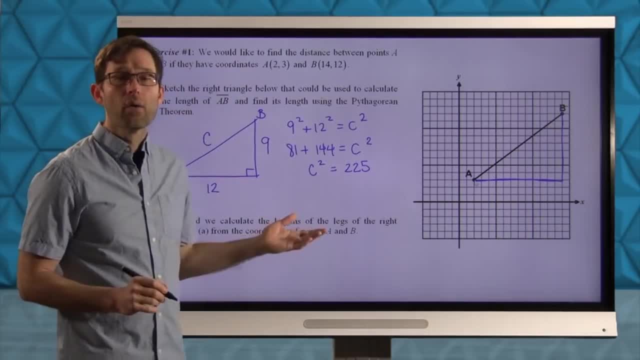 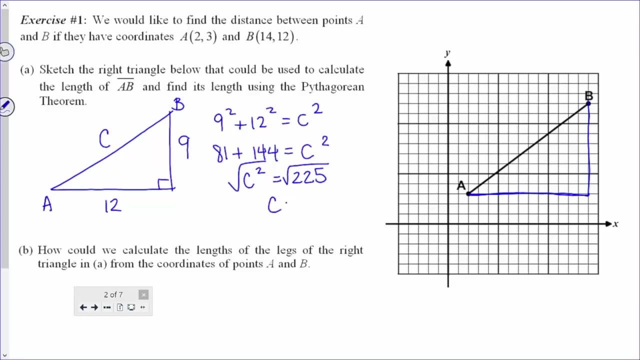 be using your calculators to do this, And then when we add those two together, we'll get C. squared is two hundred and twenty-five. Now, two hundred and twenty-five is a nice, perfect square. So when I take the square root of both sides, I find that the length of AB is fifteen, or the distance between: 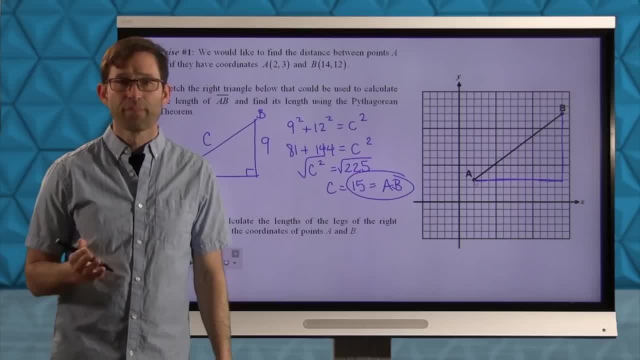 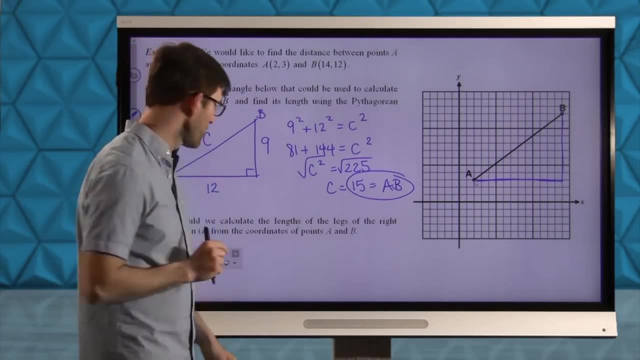 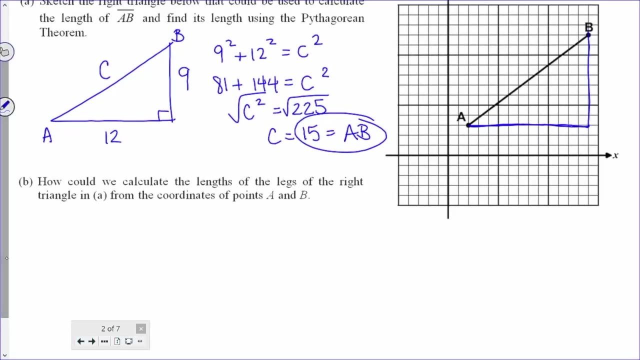 AB and B is fifteen units. Alright, Now, equally important, as this is the second part of this problem. So let's take a look at that. Letter B: How can we calculate the lengths of the legs of the right triangle on A from? 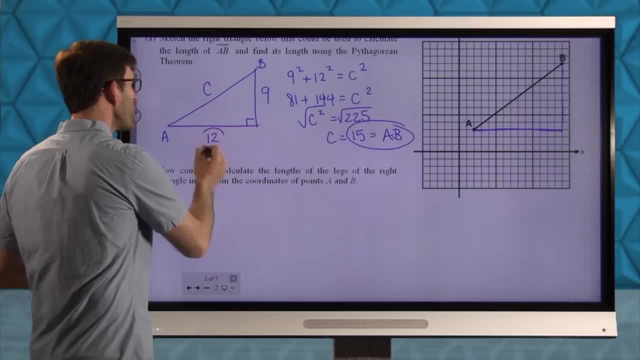 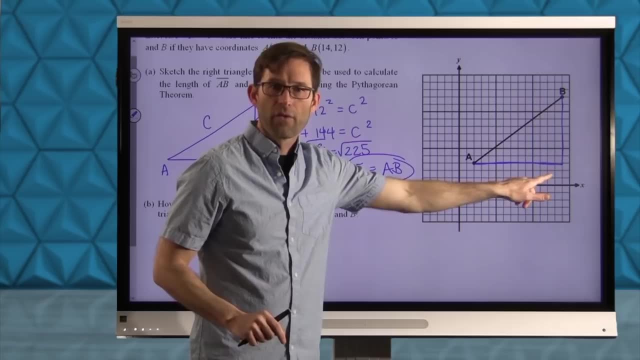 the coordinates of points A and B, in other words, I'd like to figure out. I just counted right and I literally said, okay, I've got 3, I've got another 5,, I've got another 4, so I've got 9.. Then I or sorry, so I have 12.. Then here I had 2,. 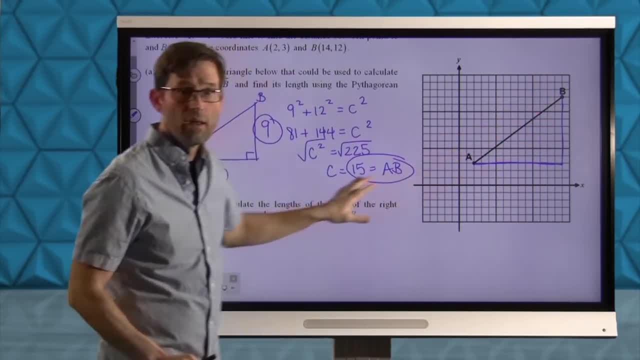 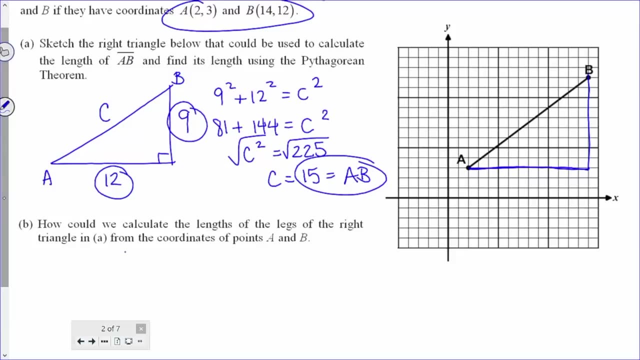 I had another 5, so that's 7, another 2, that's 9, right, But somehow I'd like to be able to use these two things. Let me bring them down. We've got A at 2 comma 3.. Hey look, my mystery red. 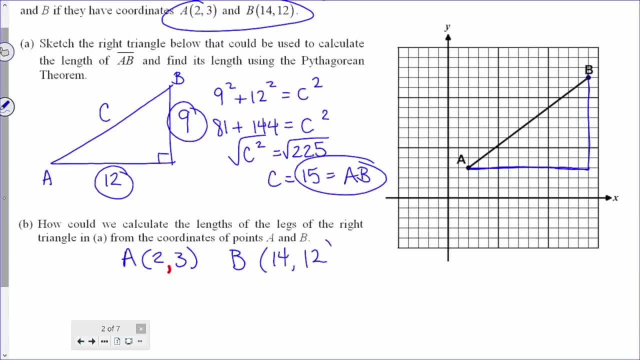 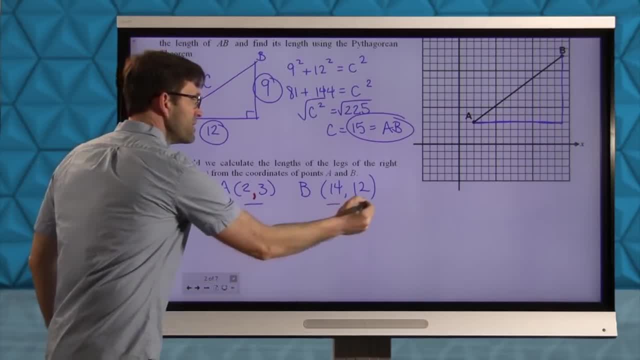 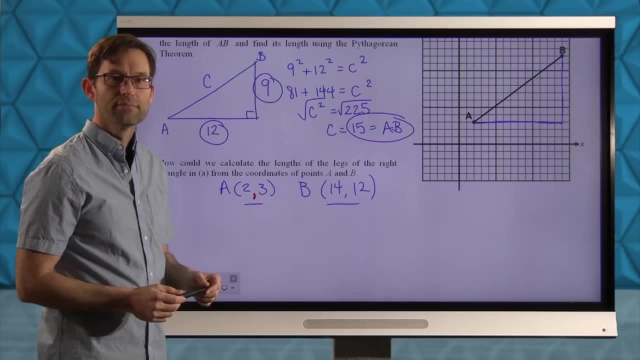 showed up. I've got B at 14 comma 12, right. How in the world can I figure out that 12 and that 9 from these two coordinates? Take a moment and think about this. All right, let's talk about it. Well, hopefully you noticed the following. 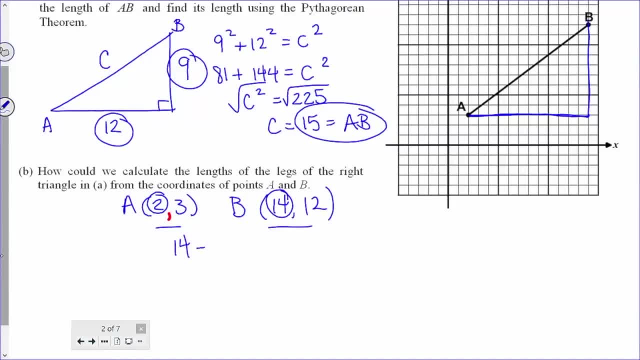 If I take these two x-coordinates and I subtract them 14 minus 2, I get 12.. And if I take these two x-coordinates and I subtract them 14 minus 2, I get 12.. And if I take these two x-coordinates? 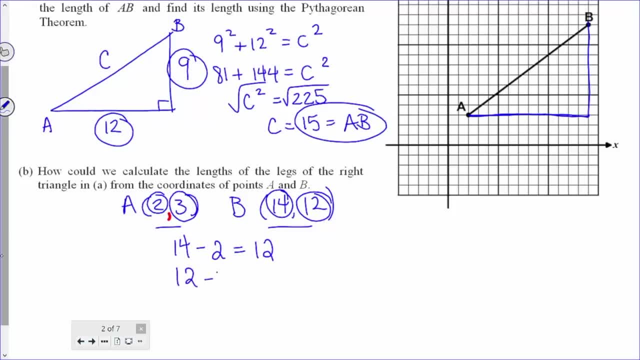 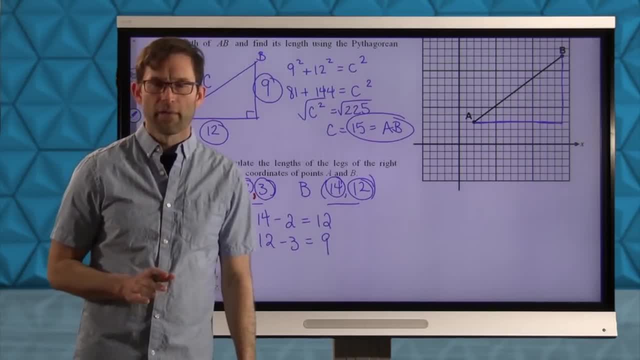 and I subtract them 14 minus 2, I get 12. And if I take these two x-coordinates and I subtract them right, I get the 9. And I hope that makes sense to you. But let's talk about it for a minute. 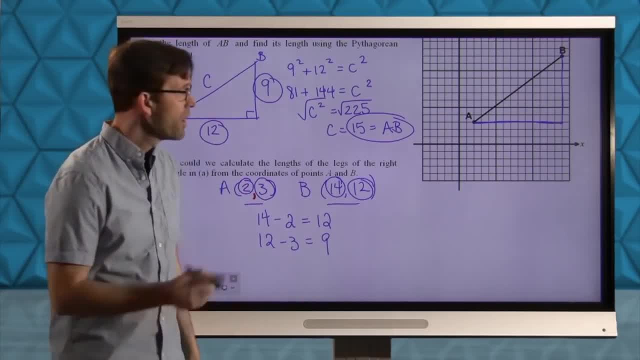 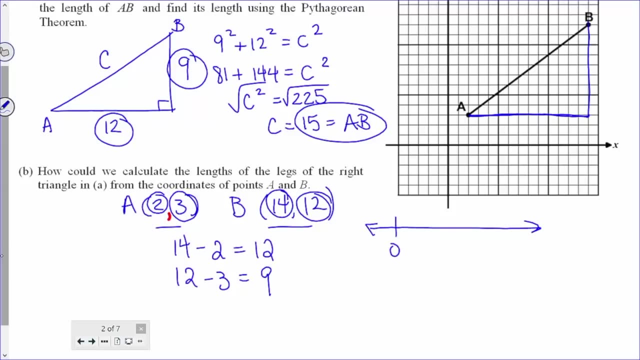 because this also comes up in the slope formula- right? Forget about two dimensions, Just think about one dimension, right? Let's say I've got this number line, okay, And I've got this number line. let's say that I had. let's switch over to red. Let's say I had a point here at 2, and I had a point. 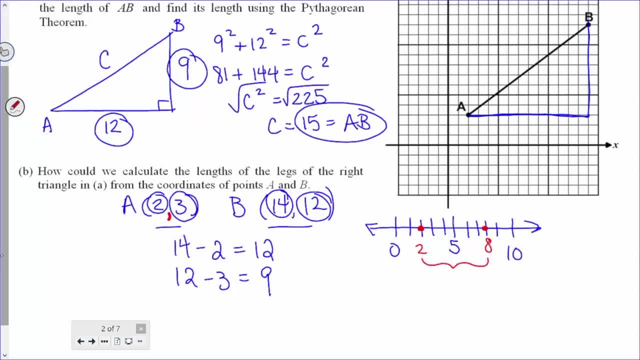 here at 8.. And I wanted to know the distance between them. all right, Sure, you could count 1,, 2,, 3,, 4,, 5, 6.. But the plain fact is what it means for that to be two units is that that's got. 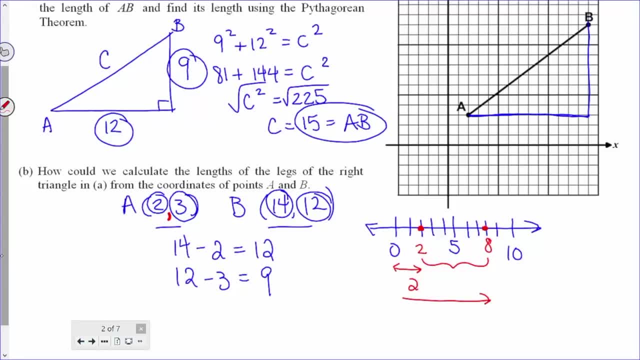 a length of 2.. And what it means for that to be 8 is that's got a length of 8.. And what it means for that to be 8 is that that's got a length of 8.. And so if I want to know the distance between: 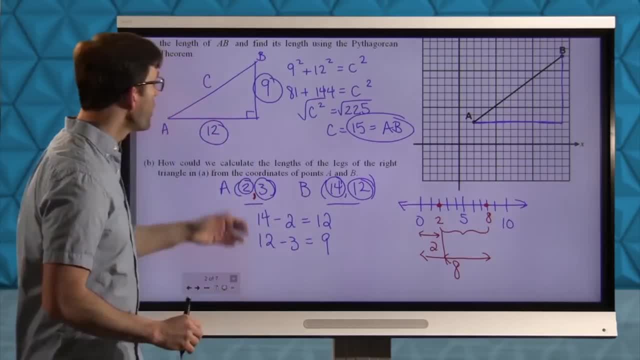 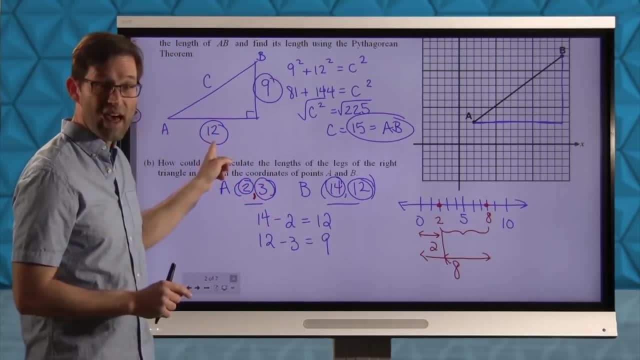 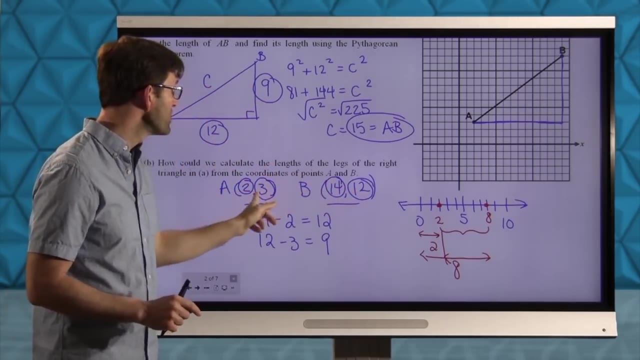 them, I simply subtract the 2 off of the 8, which is exactly what we're doing here. Whenever I want to find the horizontal distance between two points, which is that I subtract their x-coordinates, And whenever I'm looking for the vertical distance between the two points, I just subtract the y. 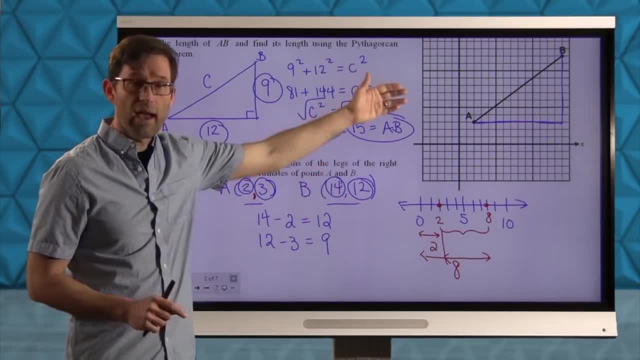 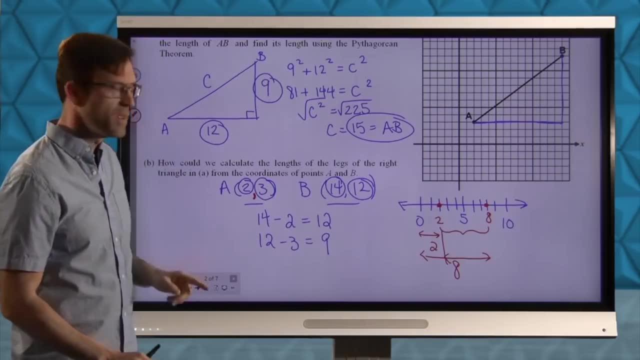 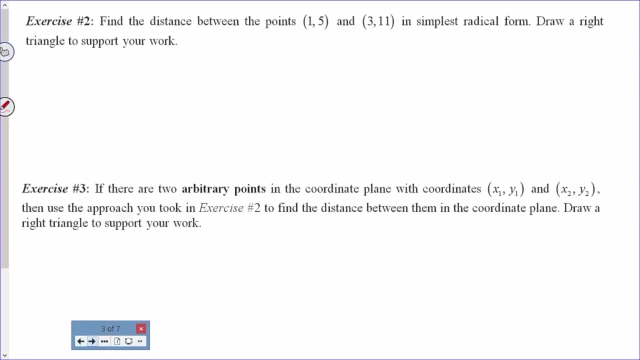 coordinates. okay, So without having to count, I can actually come up with the lengths of the two legs of the x-coordinate, The right triangle, And let's test that in the next exercise. okay, Exercise number two: Find the distance between the points 1, 5, and 3, 11, uh-oh, in simplest, radical form. Simplest radical form. 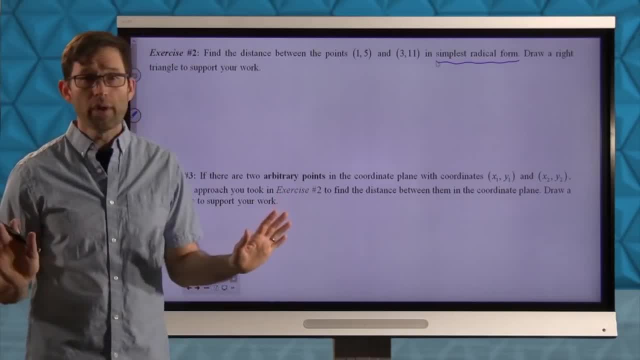 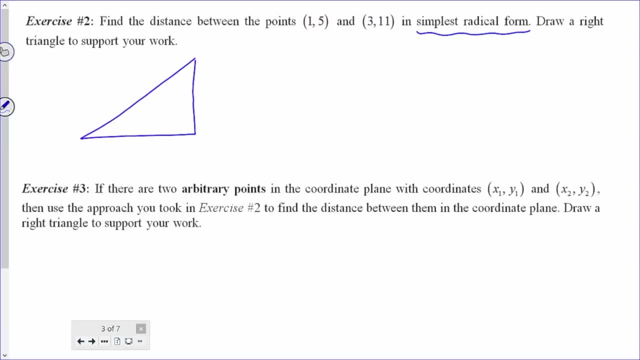 Draw a right triangle to support your work. okay, So no grid paper here. all right, No grid paper. The plain fact is, though, right, If I've got my right triangle- and I want to know how far this is- I simply take the two x-coordinates and I subtract them, right? 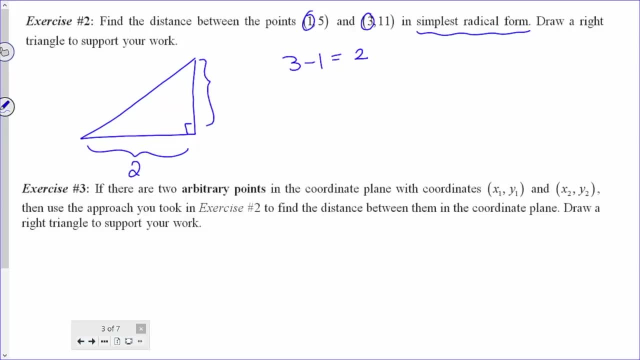 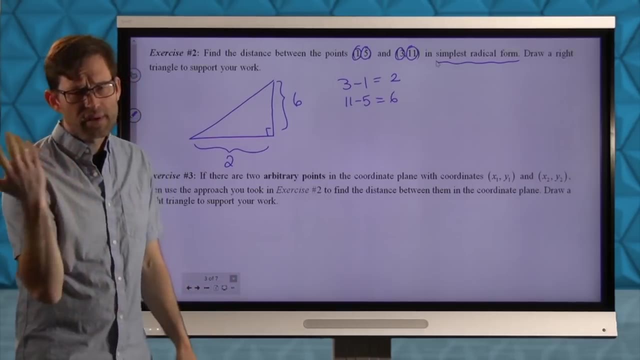 There's two units there And if I want to know this length picture not drawn to scale, I take the two y-coordinates and I get this distance. okay, Again, if we had a grid, sure plot, the two points count, if you'd like. 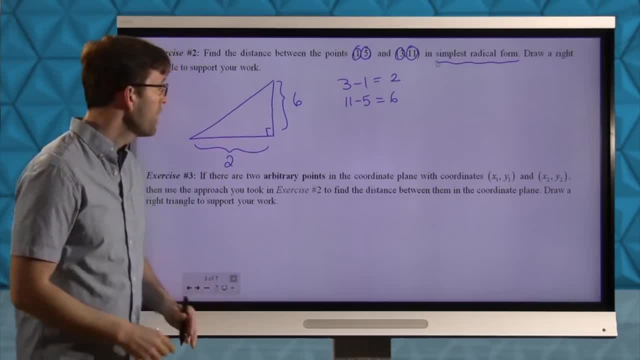 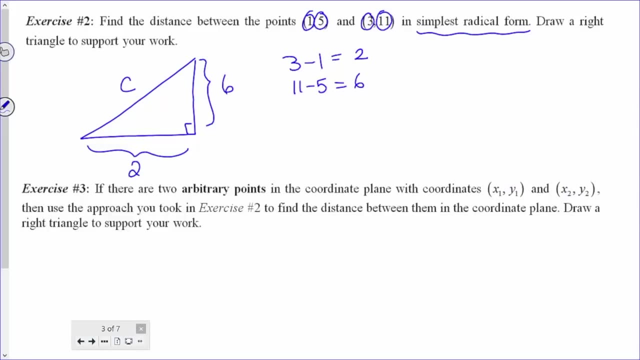 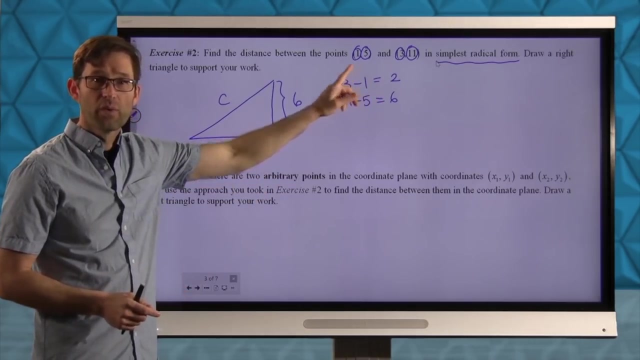 but you've got to be able to do it without counting, Okay, In which case, if I now want to find the distance between them, I do the Pythagorean Theorem. Why don't you finish that up? All right, let's go through it. And again, another further complication. we've got to get that thing in simplest, radical form. 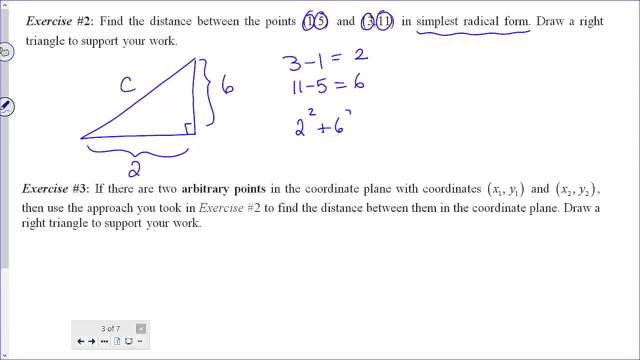 Here we go. 2 squared plus 6 squared is equal to c squared. That's 4 plus 36 is equal to c squared. c squared is equal to c squared. c squared is equal to 40.. So c is the square root of 40.. 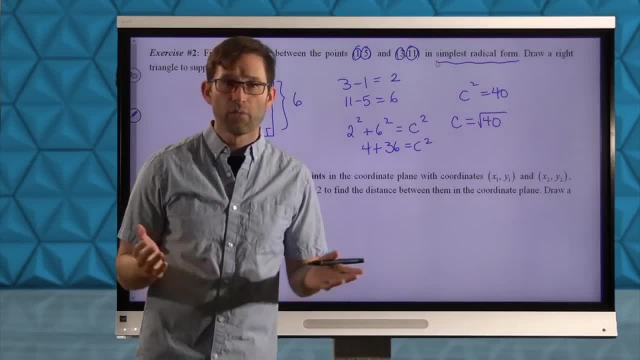 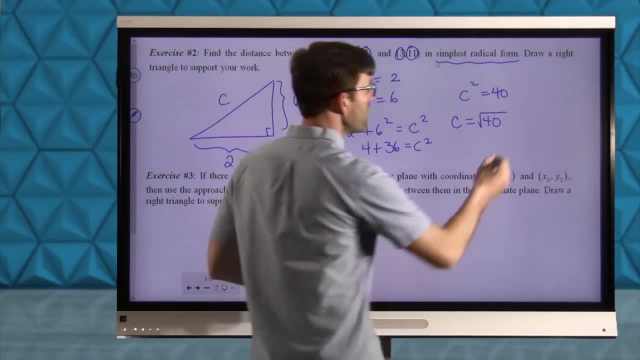 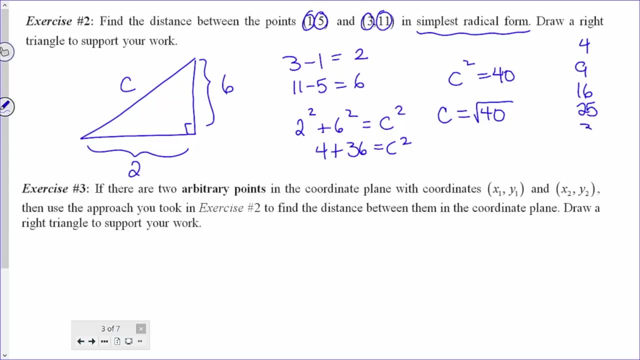 Unlike the square root of 225,, which is a nice number, the square root of 40 is not a nice number. Remember to write a number in simplest, radical form. What you're looking for is: you're looking for the biggest perfect square that fits into this number, that divides into it nicely. 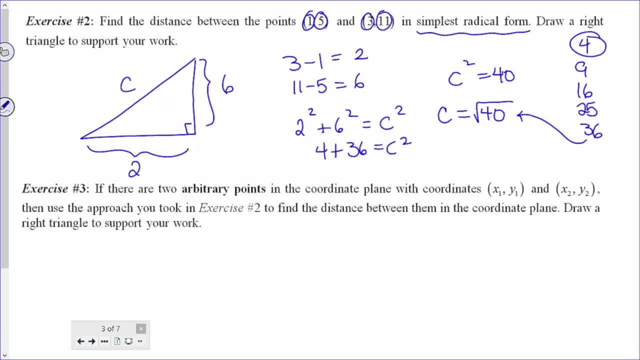 In this case, that's fairly easy, It's just 4.. Let's break this up as the square root of 4 times the square root of 10. And c would be 2 times the square root of 10.. All right, Simplest radical form. 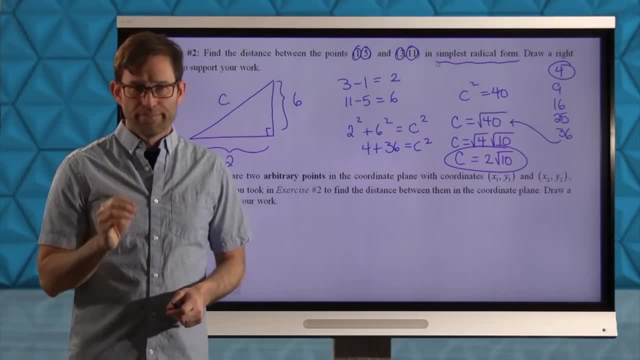 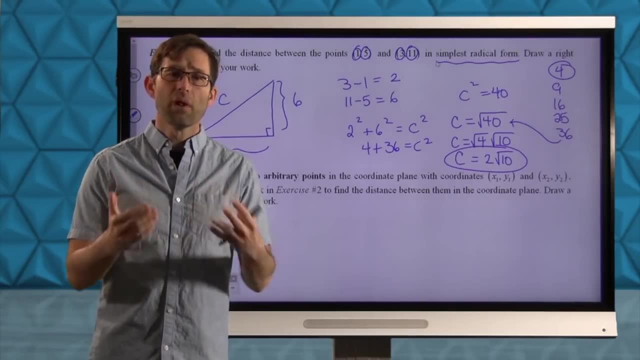 Eh, whatever Right Now. ultimately, what we would like, though, is we'd like some. I hate to put it this way, but I'm going to some plug-and-chug formula, Just like the slope formula: y2 minus y1 divided by x2 minus x1.. 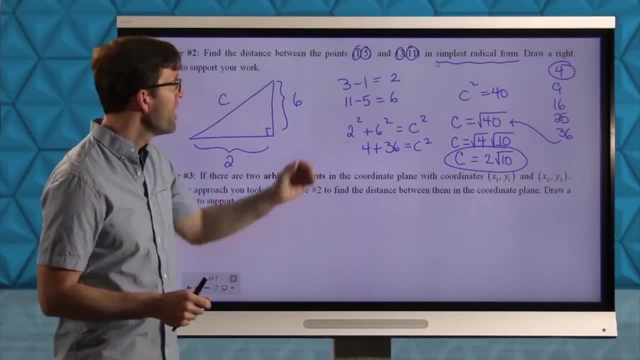 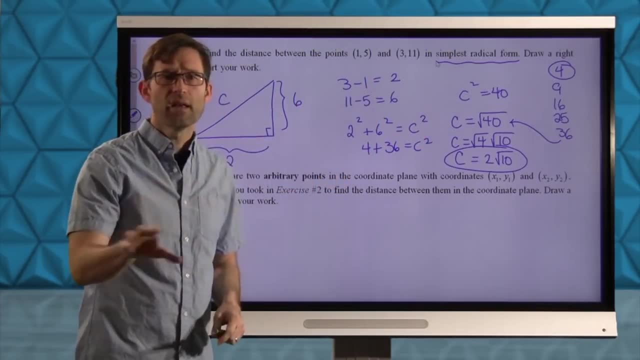 Just like the slope formula: y2 minus y1 divided by x2 minus x1.. It's a plug-and-chug formula that if I give you the coordinates, the two coordinate points, you can just kind of take the numbers, plug them in and get the answer. 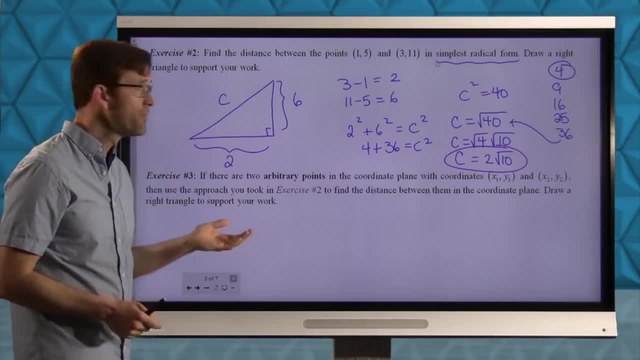 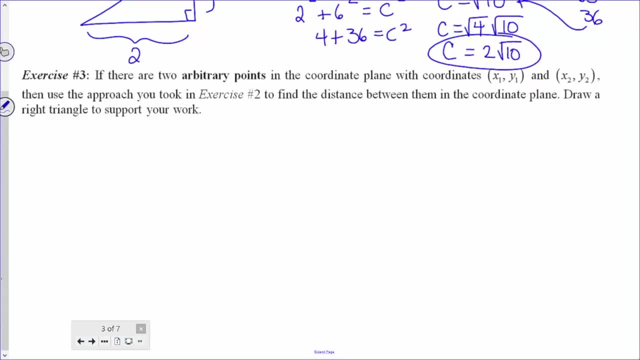 And so we're going to actually come up with that formula in exercise 3.. So what I'd like to do in exercise 3 is do exactly what I did in exercise 2, but with two arbitrary points: x1, y1, and x2, y2.. 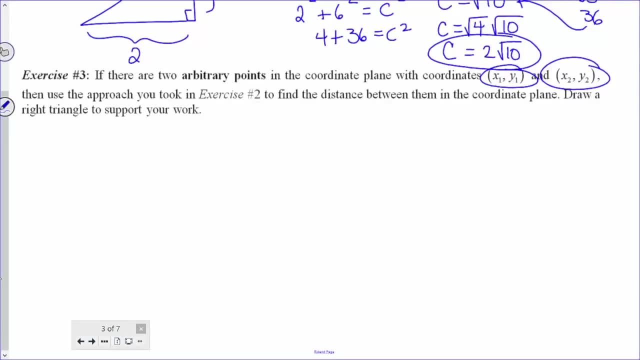 All right. So let's take a look at this, Just like before, right? The idea would be- you know the point, maybe here would be x1, y1, and the point here would be x2, y2.. All right, 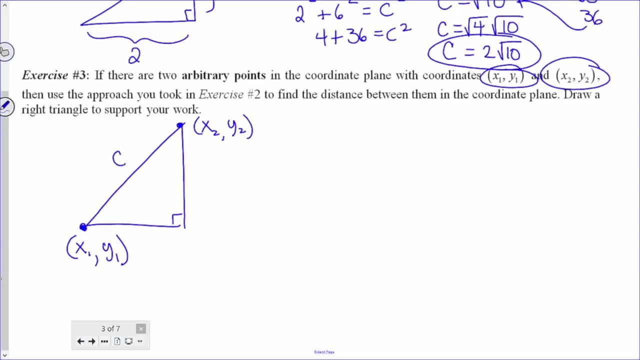 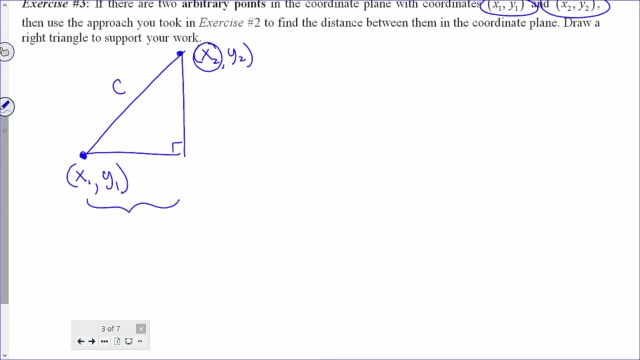 And I want to find the length of this side. Okay. Well, just based on what I did before, the horizontal length, let me extend this page a little bit. this horizontal distance will simply be this x coordinate minus this x coordinate: x2 minus x1.. 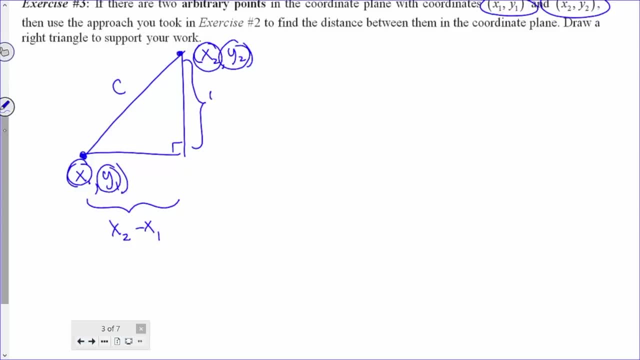 And the vertical will simply be this y coordinate minus this y coordinate, y2 minus y1.. I'm going to put some parentheses around them, okay, I'll explain why in just a moment, But then I can do the Pythagorean theorem. 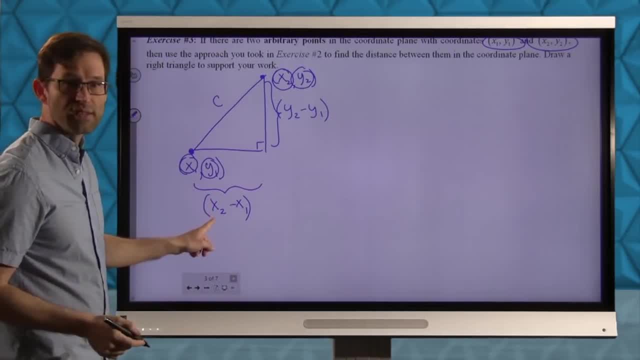 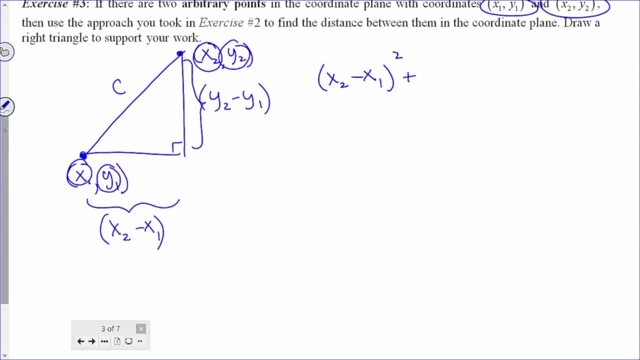 This is going to look a little bit complicated, But remember the Pythagorean theorem just says: take this distance or this length- x2 minus x1- and square it. Take this length- y2 minus y1- and square it, And then it's equal to this length. 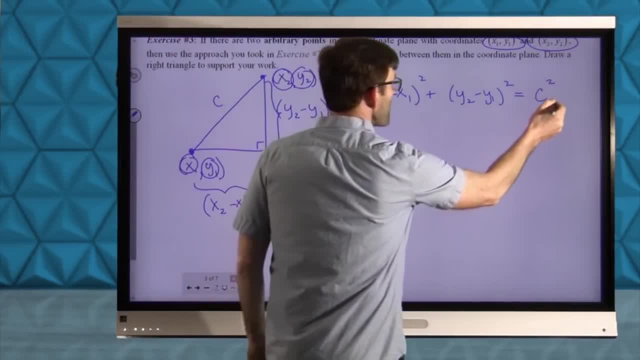 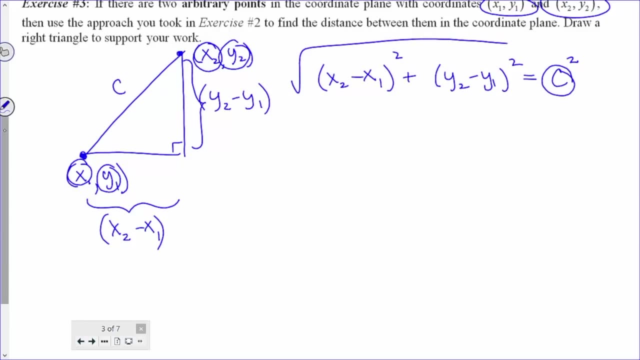 That's just the Pythagorean theorem. Now, if I actually wanted to solve for that length or that distance, I would just right now take the square root of both sides And I would find that the hypotenuse would always be the square root of x2 minus x1, squared. 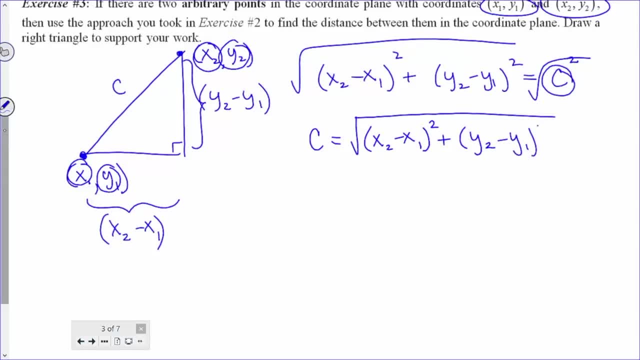 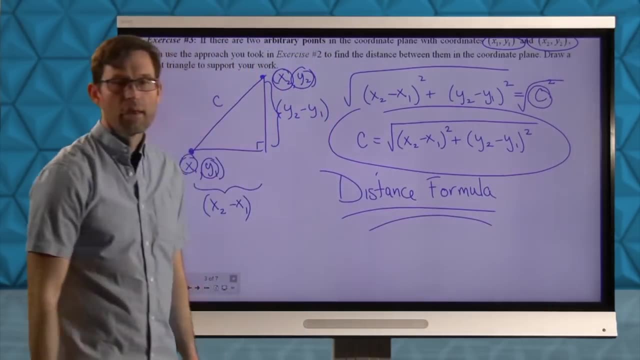 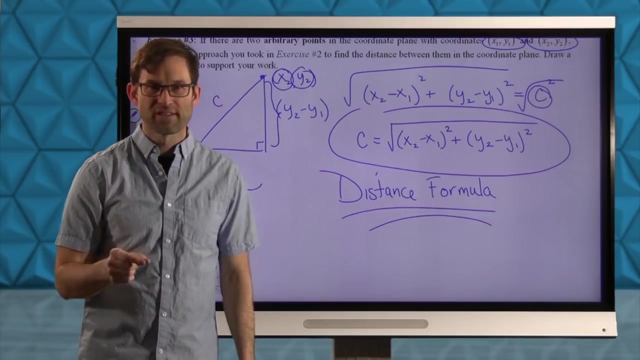 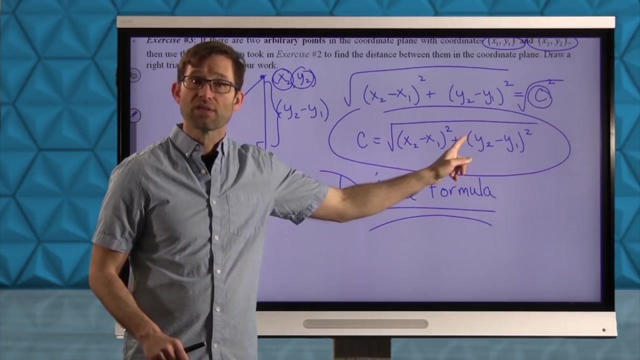 plus y2, minus y1 squared, And this is what's known as the distance formula. The distance formula is just the Pythagorean theorem using two coordinate points. Finding the difference in their x coordinates gives us the length of one leg. Finding the difference in their y coordinates gives us the length of the other leg. 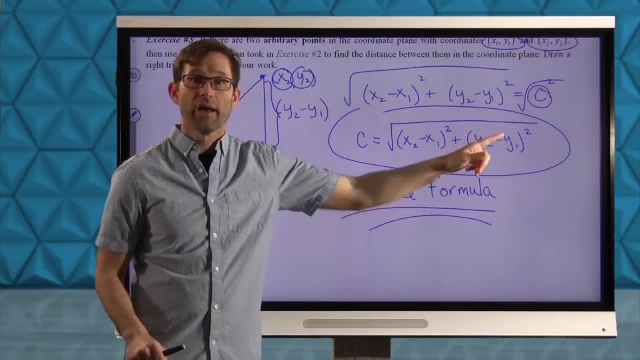 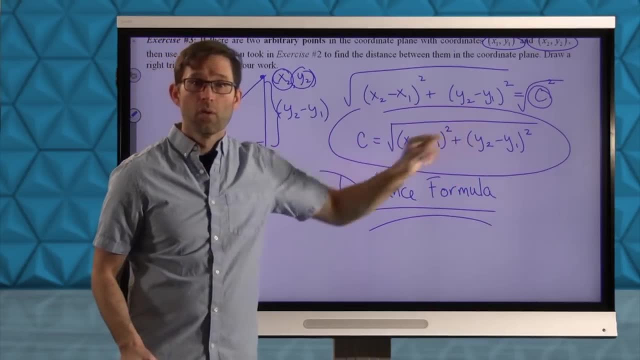 We square both of them, as we always square the two leg sides, side lengths in the Pythagorean theorem, Add it together And then, ultimately, to solve for the hypotenuse, we take the square root. Alright, That's the distance formula. 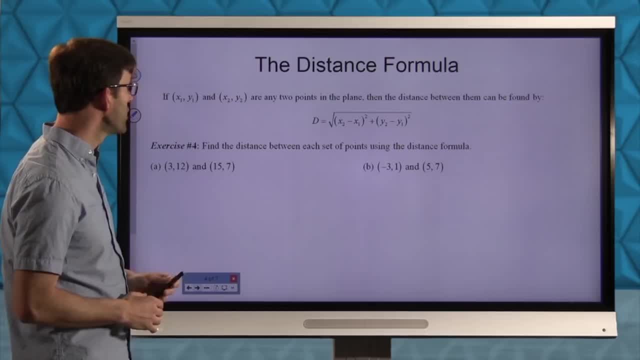 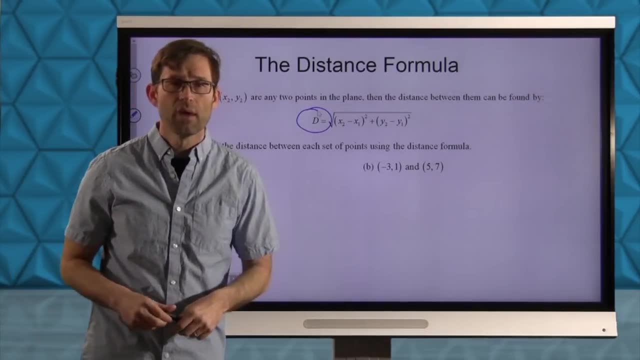 Let's summarize it in the next slide. Right Here it is. We oftentimes use a capital D for the distance formula instead of a C for the hypotenuse. One of the unfortunate things with going with the capital D versus the C is that you oftentimes then lose the fact. 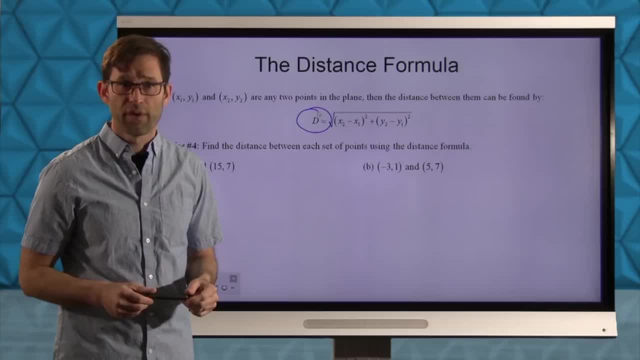 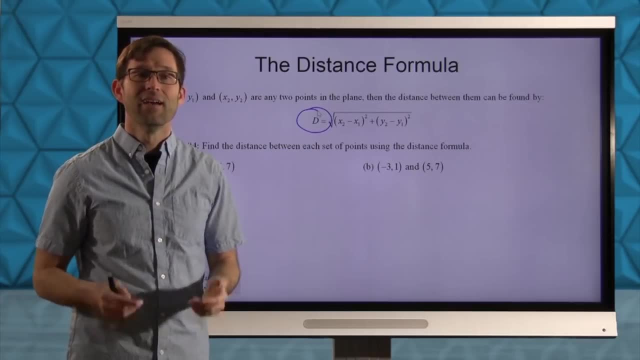 that all the distance formula is is the Pythagorean theorem. Alright, But let's get a little bit of practice with the distance formula And again, I'm going to keep going back to that idea that it's the Pythagorean theorem. 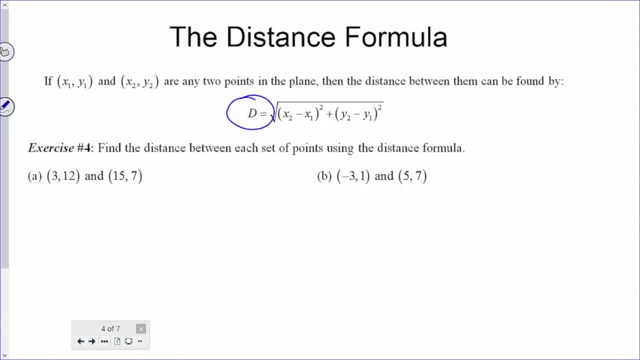 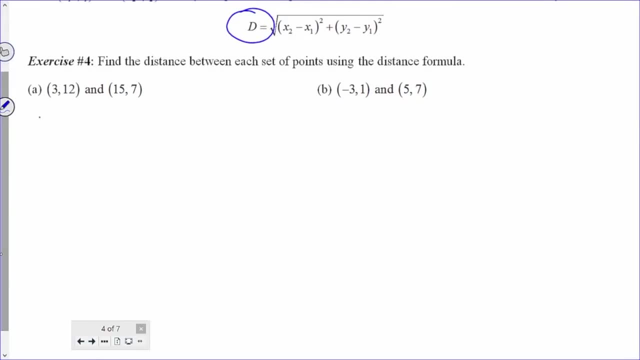 But let's take a look. Exercise number four: Find the distance between each set of points using the distance formula. Alright, So here we go, The distance formula, Right. I'm not going to rewrite it because it's sitting right up there. 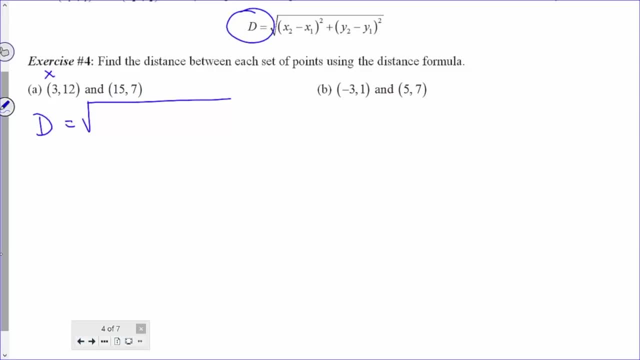 Okay, But I will maybe mark this. So this is x1, y1. And this is x2, y2.. So the distance formula says: find the difference in the x coordinates. That's 15 minus 3.. Right, 15 minus 3, which is going to end up being 12.. 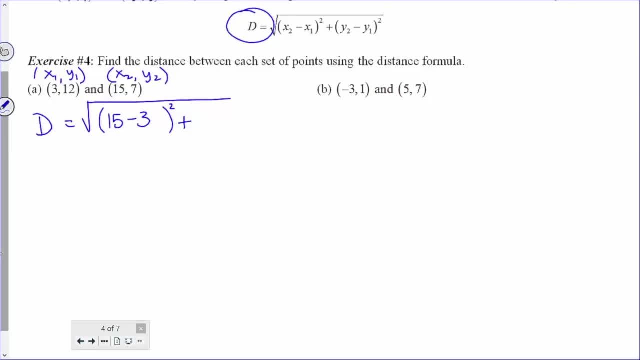 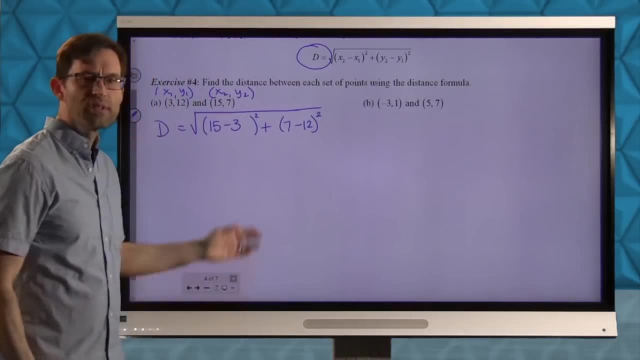 Right, That's the length of one of those legs. Then find the difference between the y coordinates, 7 minus 12.. Now, of course, 7 minus 12 is negative 5. But once we square it we get 25.. 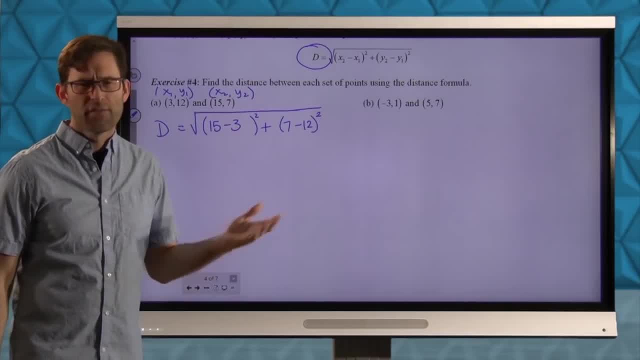 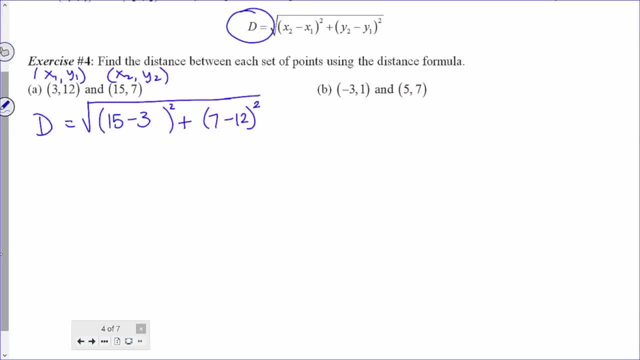 The actual length of that leg is 5.. The fact that doing the subtraction gets us negative 25, no big deal, But watch out for it when you're working on this. Watch out for it when you're working on your calculator. Alright. 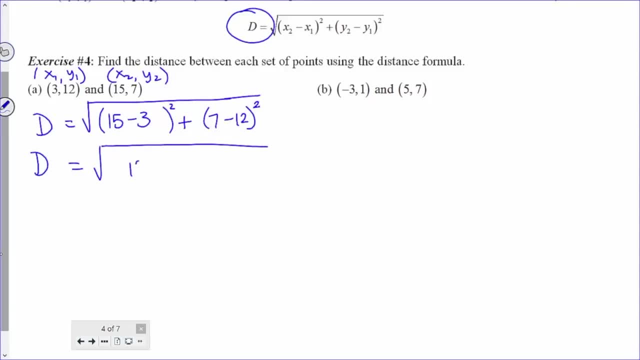 Let's kind of keep working on it a little bit, Step by step. here I'm going to get 12 squared. Here I'm going to get negative 5 squared. Alright, When I square 12, I get 144.. When I square negative 5, I get 25.. 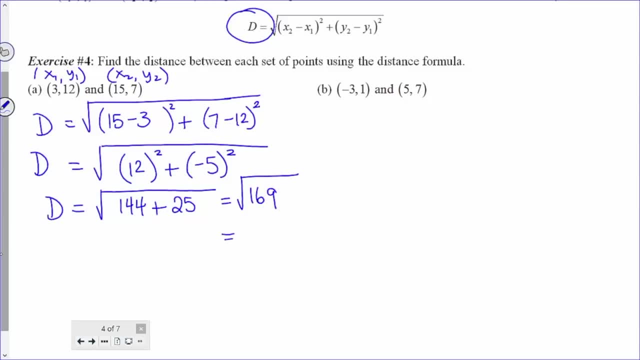 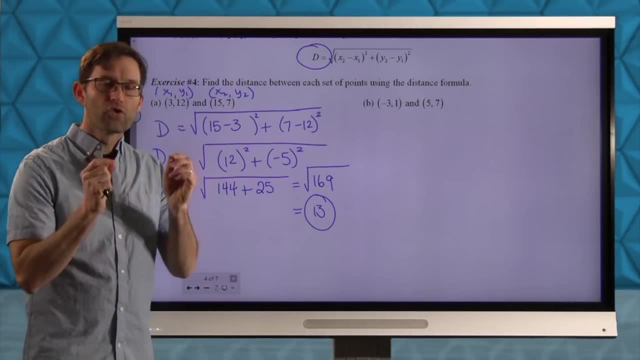 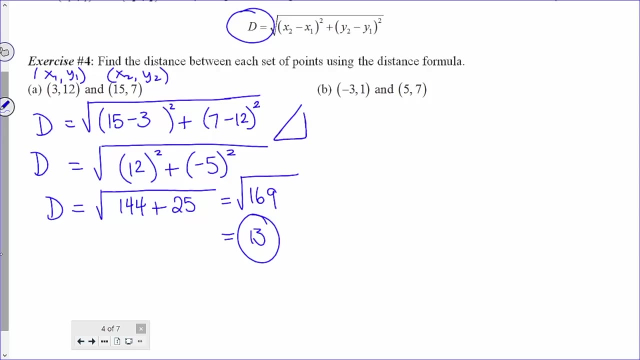 When I add them together, I get 169.. Take its square root and I get 13.. And that's it Really and truly. really and truly. we're doing nothing more than having some right triangle right that has one side length of 12,. 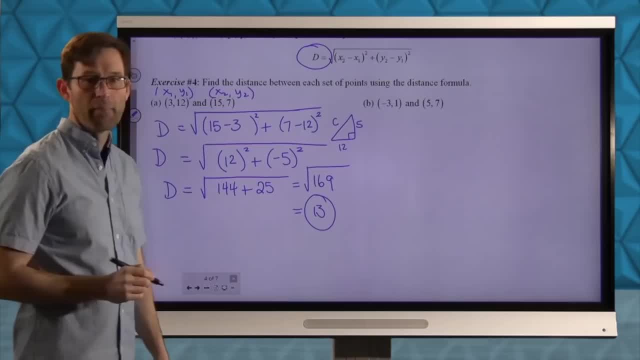 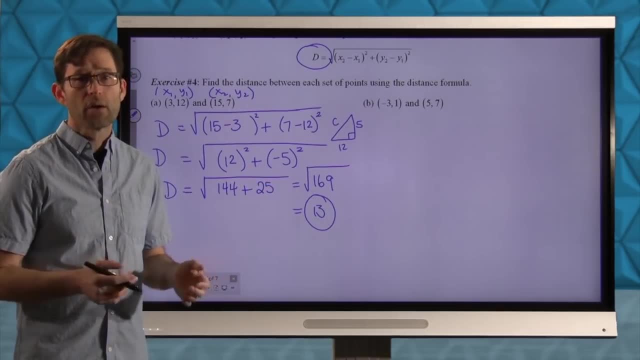 one side length of 5, and we're finding that the hypotenuse is 13.. That's all we're doing: Square, square, add. take the square root Here. one extra step. we've got a new subtraction to simply find out the length of those legs. 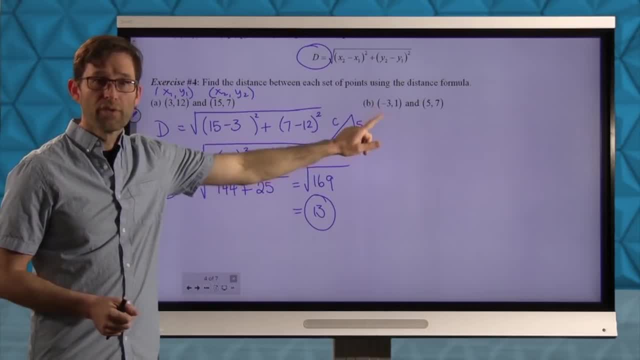 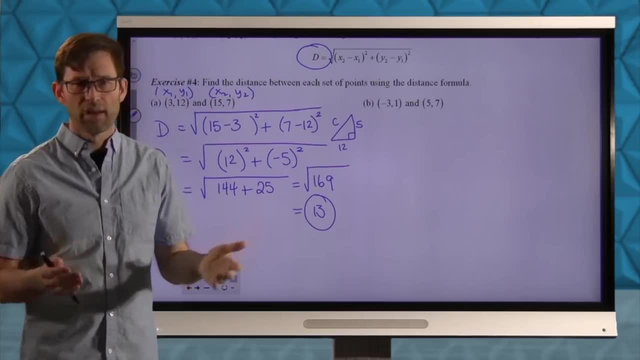 Alright, Why don't you work on problem B? Be careful, There's going to be subtracting a negative in letter B, so that can get a little bit tricky. But work through it. Your answer will come out to be nice. It'll be an integer. no simplifying radicals. 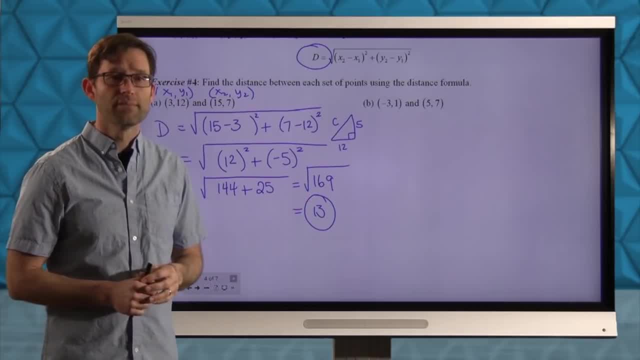 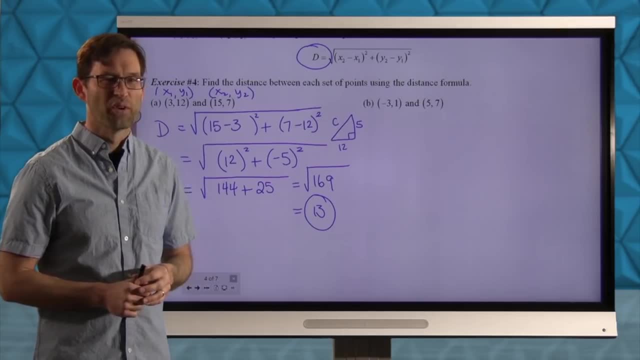 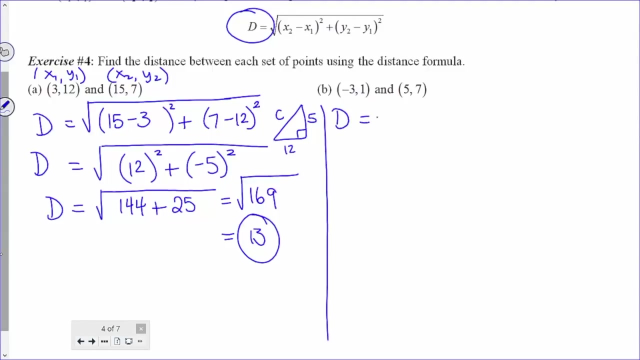 or anything like that here. So go ahead, Take a few minutes. Alright, Let's work through it. I never know what to do in those pauses. Alright, The distance for a line. Alright, The square root of let's take 5 minus negative 3,. 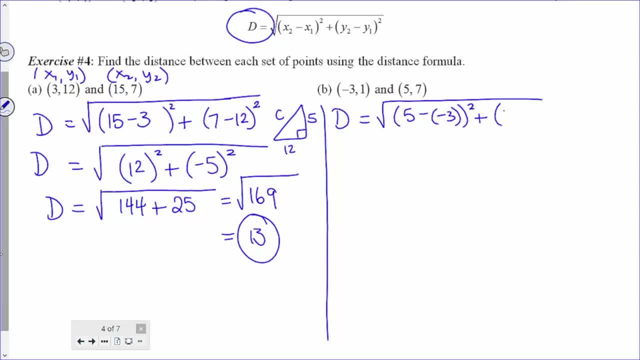 just be careful on that. one squared plus 7 minus 1, squared Alright. Again, you've got to be careful here. The distance between negative 3 and 5, between that x coordinate of negative 3 and that x coordinate of 5,. 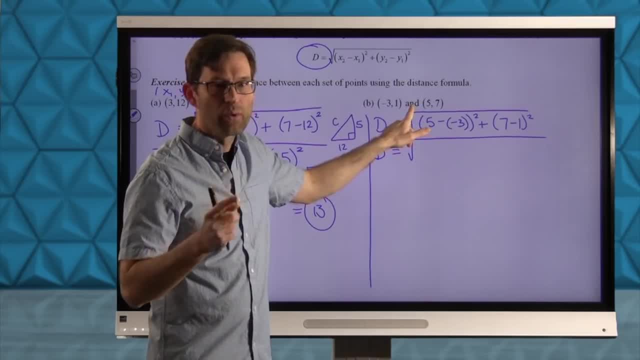 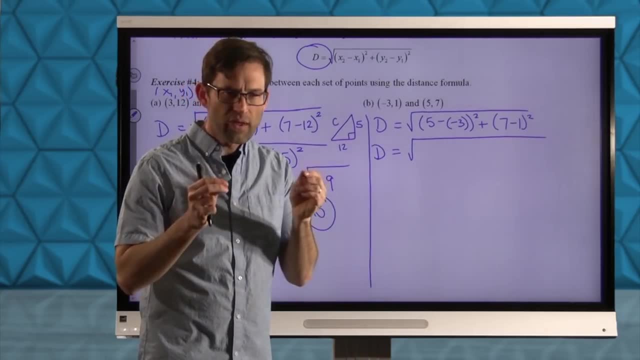 is 8 units, It's not 2 units, and you know that Right. So don't do 5 minus negative 3, and get 2.. It's just not the case. Think about what you're doing. You're calculating a distance. 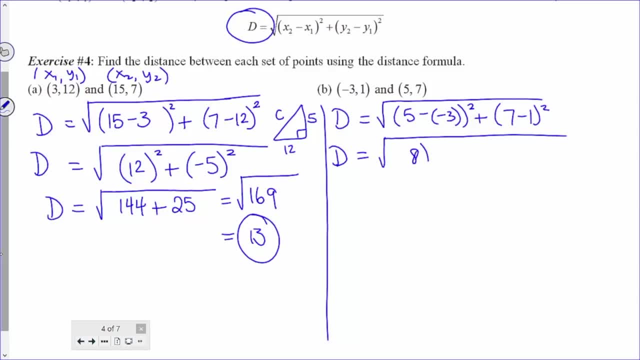 Anyway. So what do we get? We get 8 squared. Here I'll get 6 squared. So we get 64 plus 36.. Add those together we get 100.. The square root of 100 is a nice number. 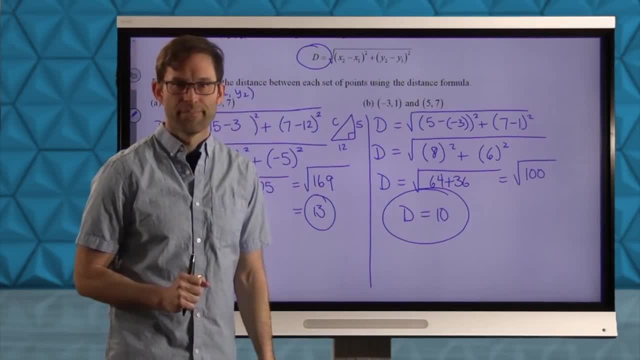 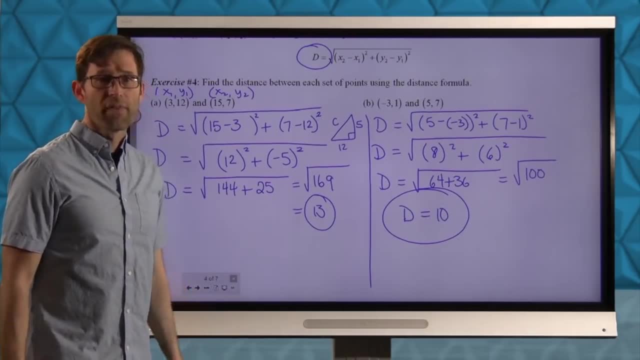 And we find that the distance is 10.. Alright, That's it. The distance formula is actually fairly easy to use. Again, it's just like the Pythagorean theorem. The nice thing is, you're always solving for the hypotenuse. 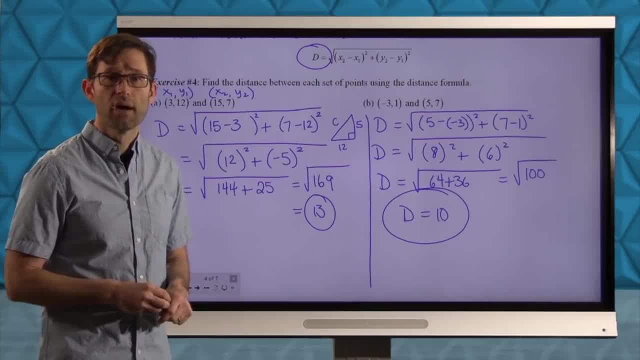 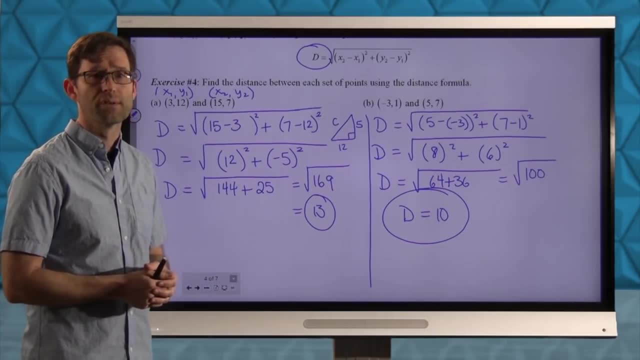 You're not solving for one of the legs. That's kind of nice. Anyway, Take a little bit of time, Write down anything you need to, and then we'll work some where the answers are a bit messier, But we're still just using the distance formula. 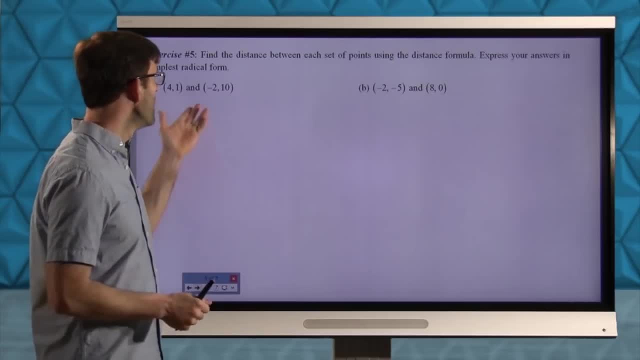 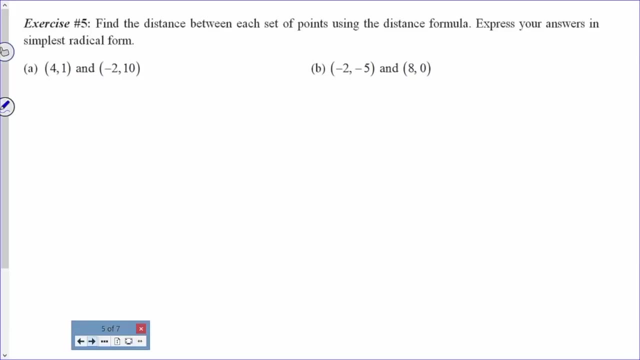 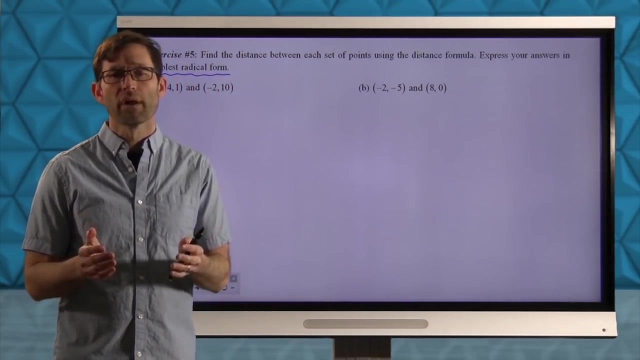 Alright, Let's move on. Okay, Exercise 5. Find the distance between each set of points using the distance formula. Express your answers in simplest, radical form. Alright, So exactly the same procedure that we had before, except now we're going to expect our answers to be a little bit messier. 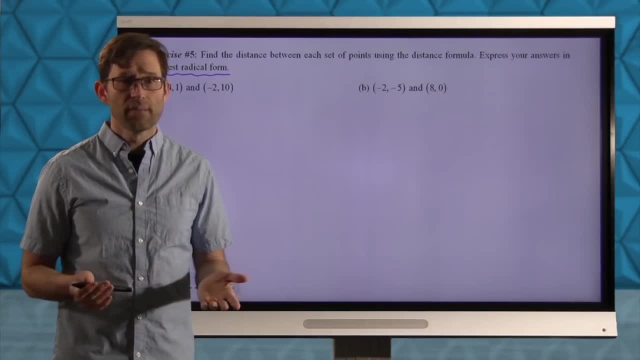 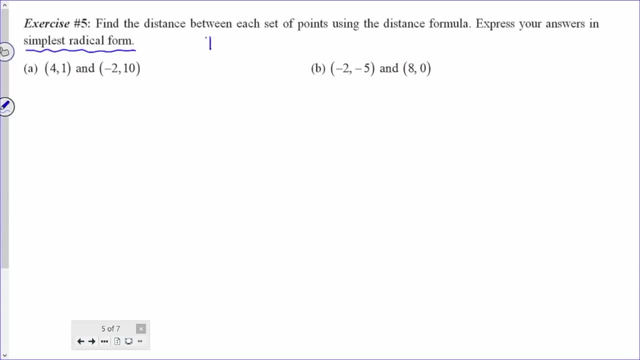 and we'll have to maybe work with simplest radical form, But that's it. So let's take a look at the first problem together and we'll have you work on the second one on your own. Let me write out the distance formula. 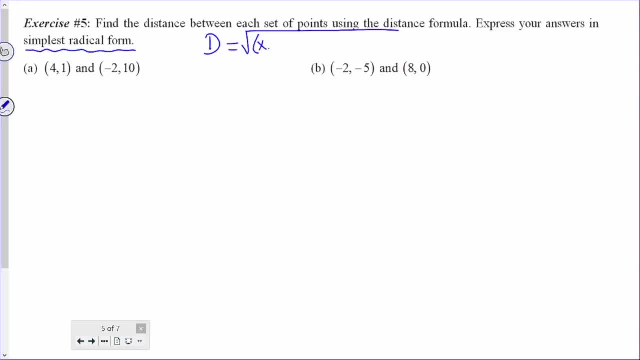 I'll write it right here: The distance formula, The square root of x2 minus x1 squared. That doesn't look like a square y2 minus y1 squared. Let me add a little loop there. Okay, That looks a little bit better. 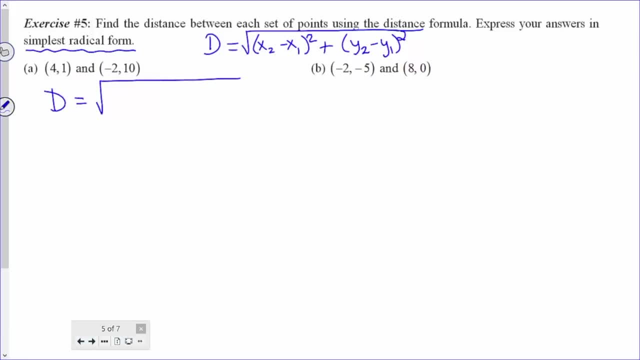 Alright. So first problem, The distance is the square root of negative 2 minus 4 squared- That'll be a little bit tricky- And 10 minus 1 squared. And just be faithful And do step by step. Negative 2 minus 4 is negative 6.. 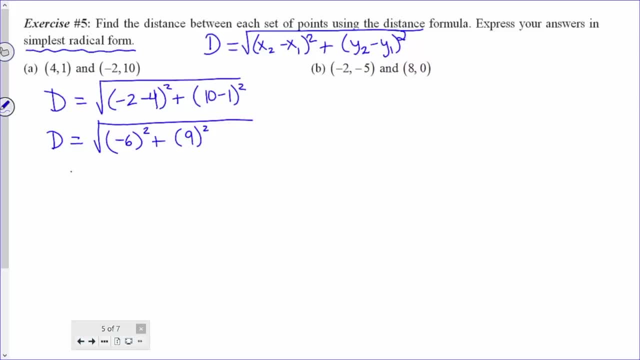 10 minus 1 is 9.. Remember that whenever you square a negative, it becomes a positive. So, negative 6 squared is 36.. Obviously, 9 squared is 81.. And then we get the square root of 117.. 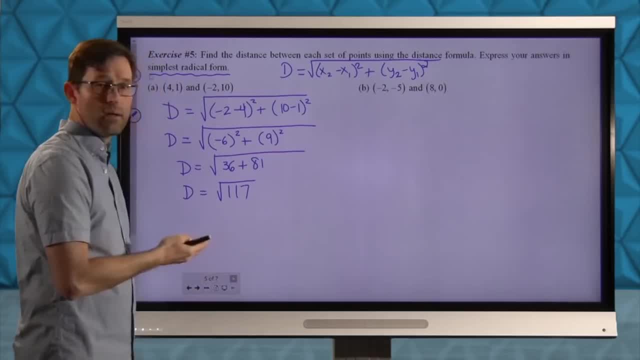 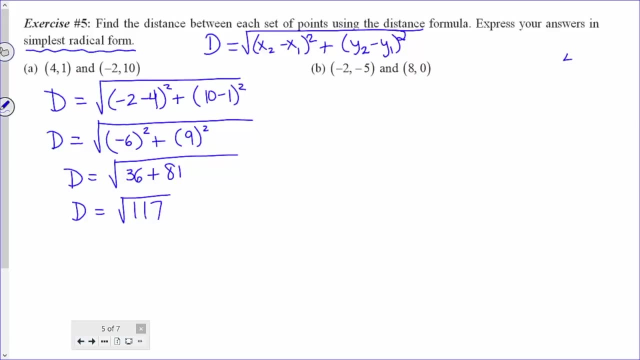 Now the square root of 117.. The square root of 117.. The square root of 117 is not a nice number. It may also not be obvious to you which, if any of these perfect squares right, goes into 117.. 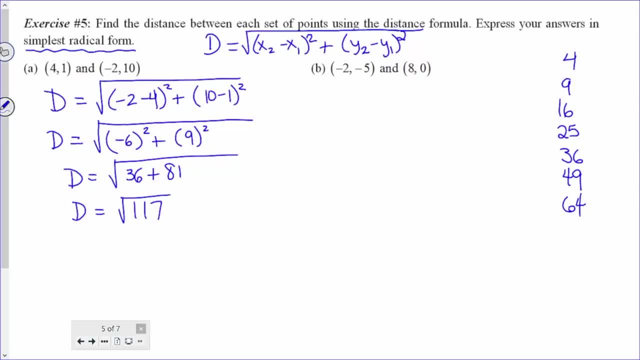 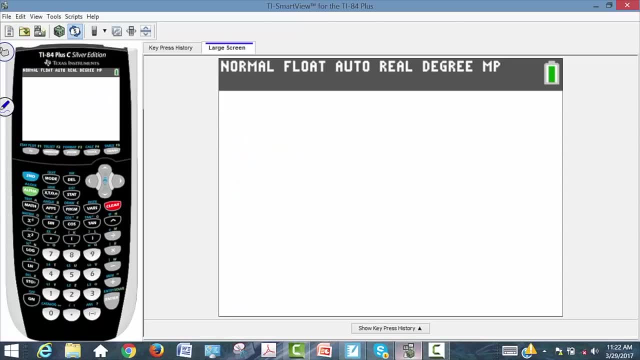 Alright, That's where, of course, it can be useful to have your calculator. So just for a moment, let me break out of this and go into my TI. Right, I'm trying to figure out what the biggest perfect square is. that goes into 117.. 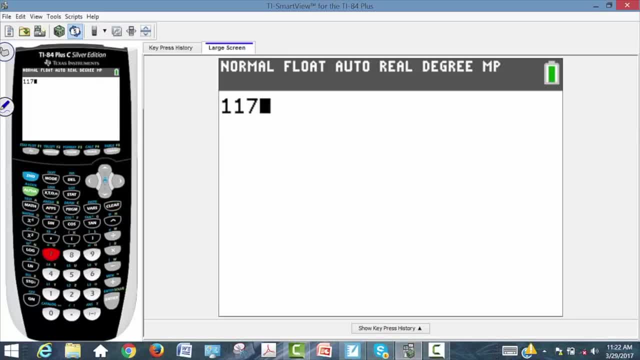 Now there's an argument that can be made that you should start with maybe some of the larger ones, like, I don't know, maybe 49 goes into it, Nope, So maybe get a little bit smaller, Maybe I can take a look at 36.. 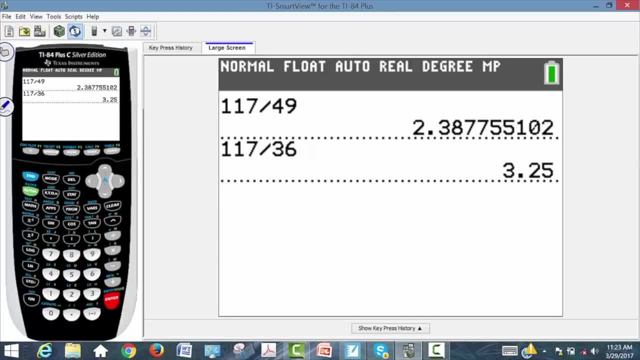 That's much nicer, but it's still not a whole number. How about 25?? No way 25 goes into that. Let me look at 16.. Still not nice. Maybe that's as good as I'm going to get. Let's try 9.. 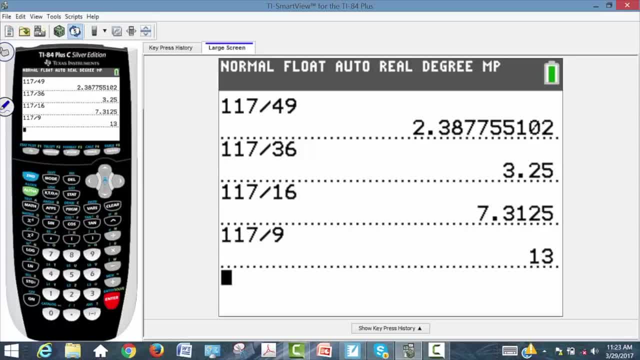 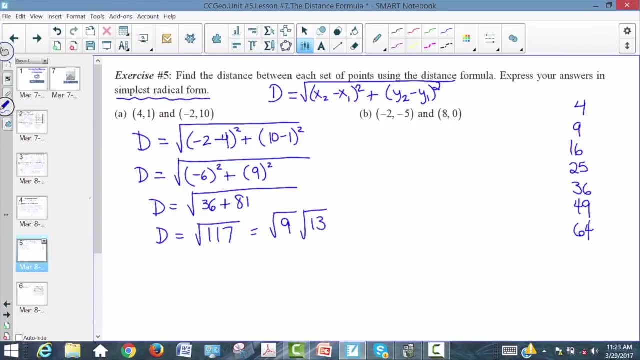 Oh there, it is Right. 9 times 13 is 117.. So 9 is my biggest perfect square. that goes into 117.. So let me kind of go back over here. I can break this up as the square root of 9 times the square root of 13,. 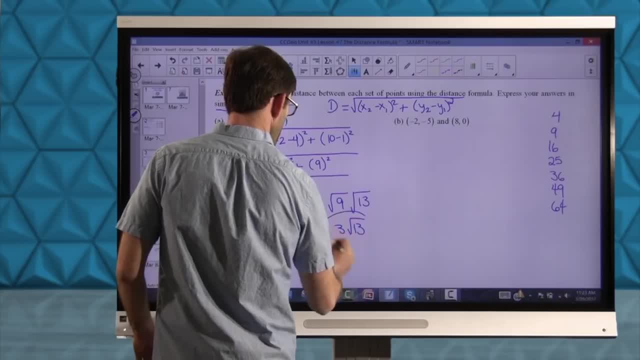 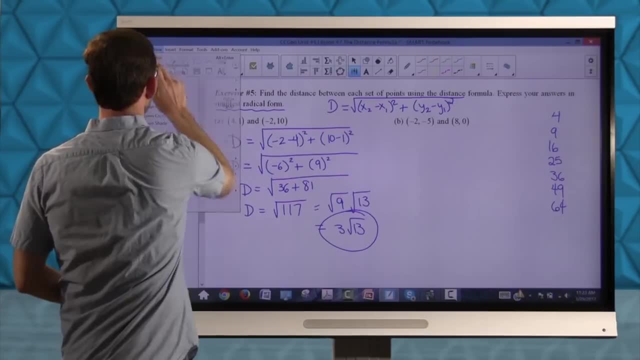 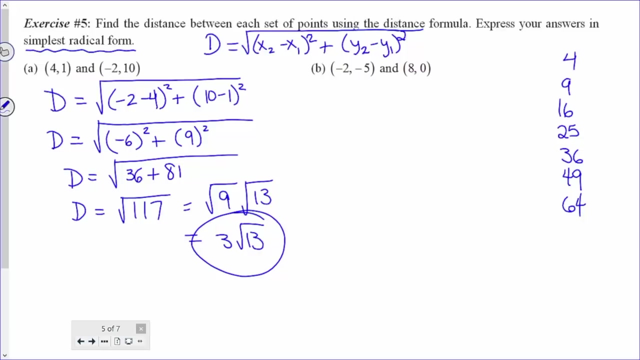 which gives me 3 radical 13,, or 3 times the square root of 13,, as my final answer. All right, Why don't you work on letter B? Take a moment? All right, Let's go through it. Ah, the distance formula, yet again. 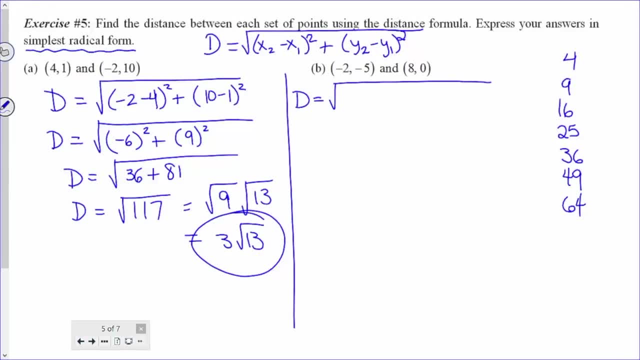 Plug and chug. plug and chug Distance is the square root of 8 minus negative. 2. Be careful there again Squared. Also, make sure you're squaring 0 minus negative. 5. Look at all the parentheses. 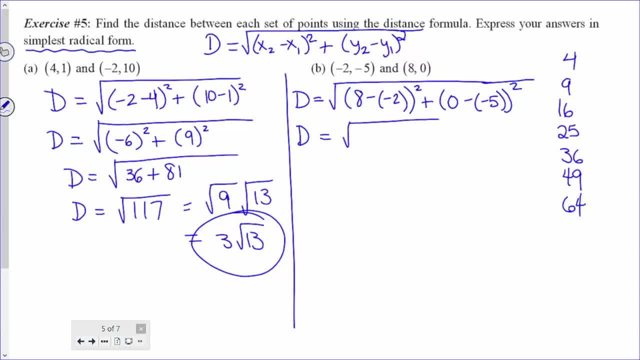 Again, watch out: 8 minus negative 2.. It would be easy to think that's 6,, but the distance between negative 2 and 8 on a number line is 10 units, not 6 units. So we have then 10 squared. 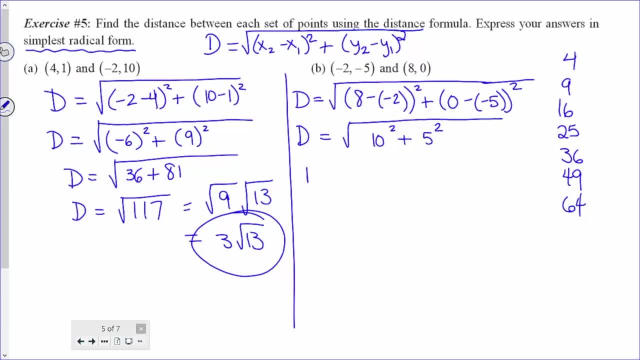 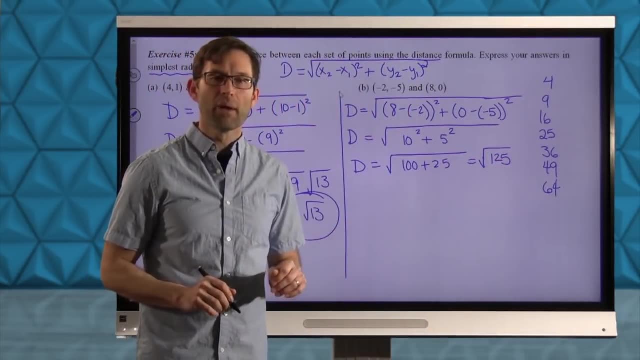 Here we'll have 5 squared, So we'll end up having 100 plus 25, or the square root. Oops, Where did that square root symbol go? The square root of 125.. Here, I doubt I'm going to need my calculator. 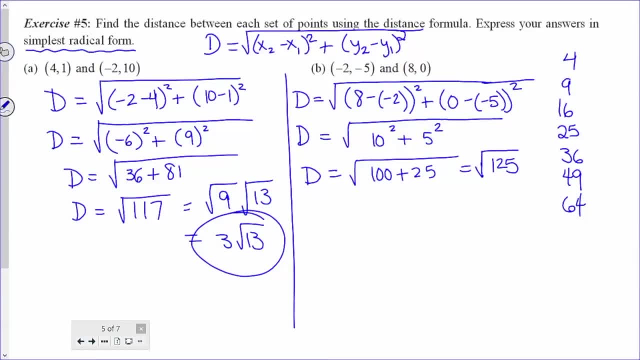 to figure out the largest square. that goes into 125.. Hopefully, it's pretty obvious that it's going to be 25.. Right, I mean it should be, And I can break this up then as the square root of 25 times the square root of 5.. 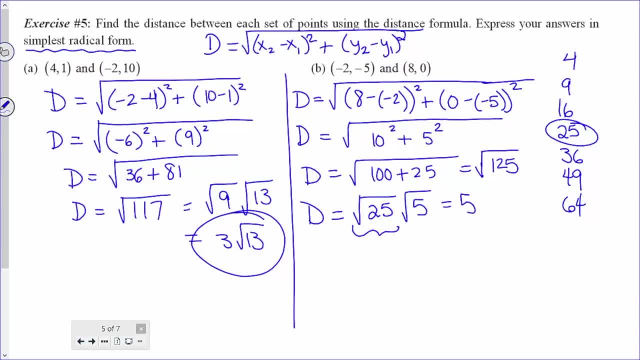 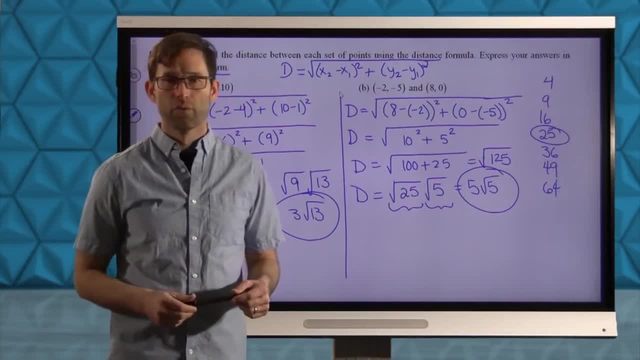 Take the square root of what you can. The square root of 25 is 5.. Leave what you can't The square root of 25.. And that's it, 5 root, 5. Okay, Now again, you know, if they don't say: put it in the simplest radical form. 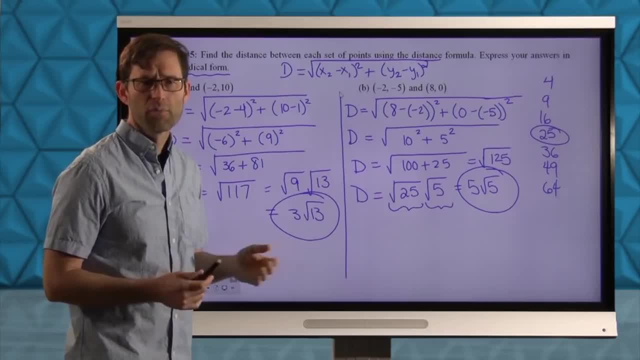 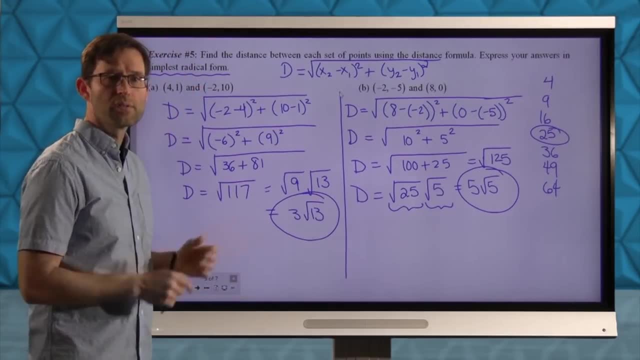 you can just kind of leave it like that, depending on your purpose, All right. So what do we have? I think we have one more problem to go. Take a look at the work, spend a little bit of time and then we'll move on to that final problem. 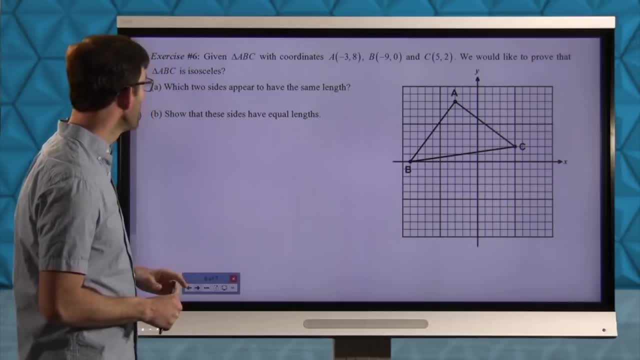 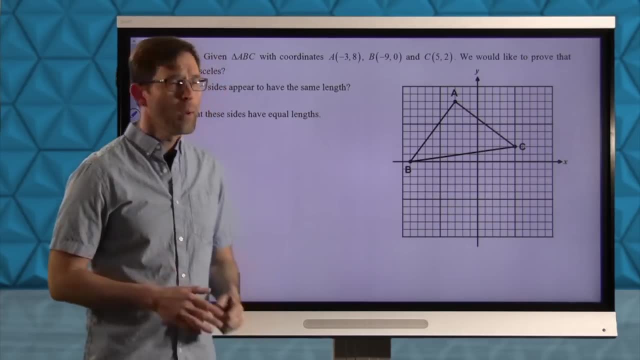 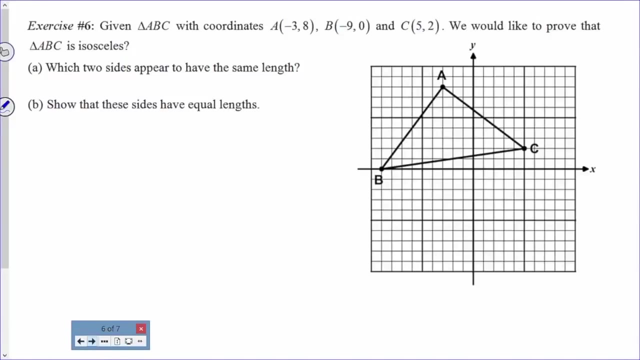 All right, Let's do it. Exercise number 6.. Now this starts to get at, ultimately, why we even need the tools of coordinate geometry. We want to prove something about the triangle plotted in the coordinate plane. Let's take a look. Given triangle ABC with coordinates negative 3, 8, negative 9,, 0,, 5,, 2,. 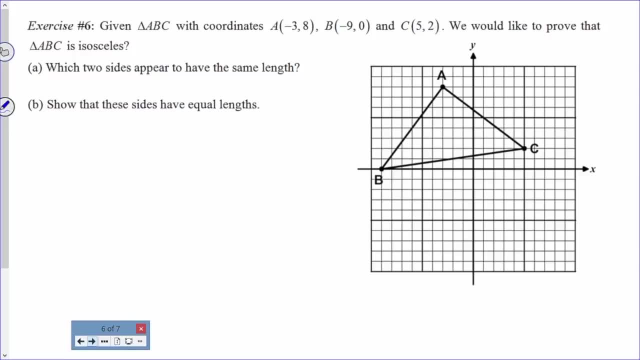 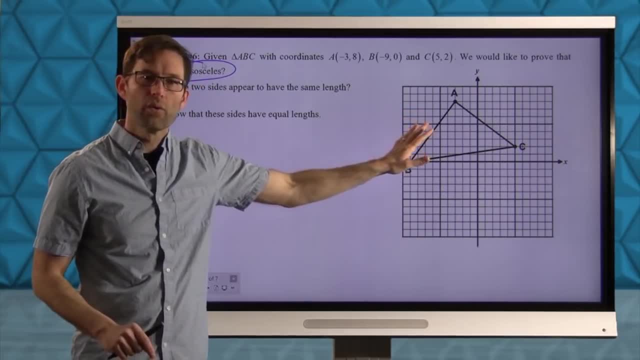 we would like to prove that ABC is isosceles. All right. Well, if the triangle hadn't already been plotted for us, we'd want to do it right now. But it's there, It's sitting there, I don't need to plot it. 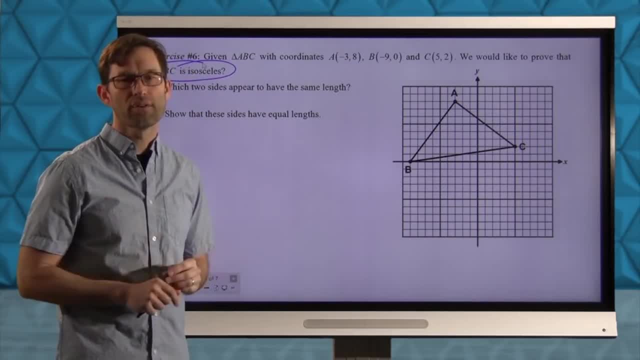 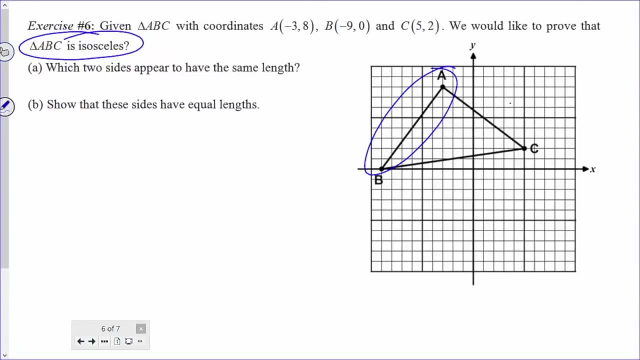 Okay, Letter A, Which two sides appear to have the same length. Well, it kind of looks like AB and AC. So it kind of looks like side AB and side AC appear to have the same length. Letter B Show these sides have the same length. 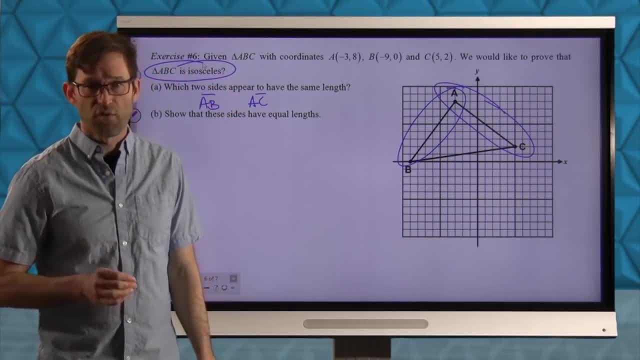 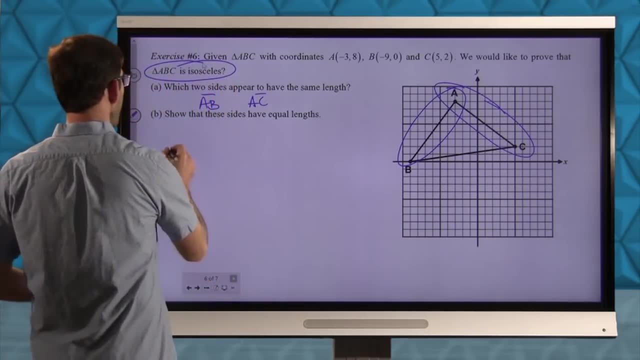 Well, the way I'm going to do that is by using the distance formula, All right, And I just have to be systematic about it, Okay, So let's take a look at AB together and then have you do AC on your own. 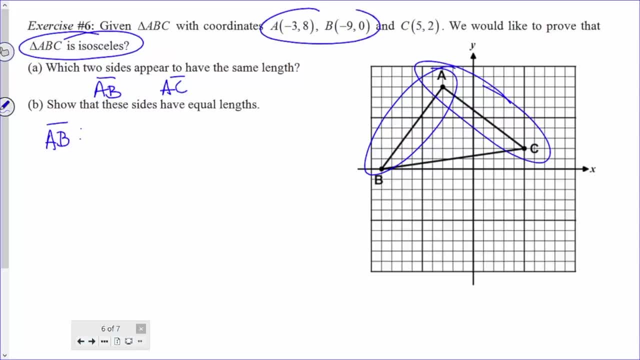 Hopefully you'll get the same answer. So for AB I've got to take these two coordinates and use that distance formula. So I'm going to say that I've got negative 9 minus negative 3, again, be careful there. 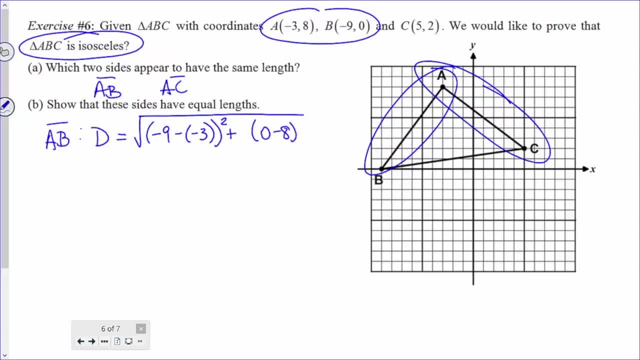 squared plus 0 minus 8 squared- Watch out here: Negative 9 minus negative 3 ends up being negative 6.. 0 minus negative 8, that's easier, That's just negative 8.. Be careful about squaring negatives. 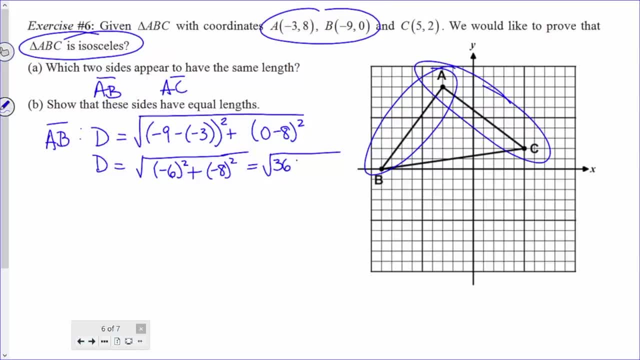 They always turn positive. Negative 6 times negative, 6 is positive 36.. Negative 8 times negative: 8, positive 64. That ends up giving me the square root of 100.. So it looks like AB has a nice length of 10.. 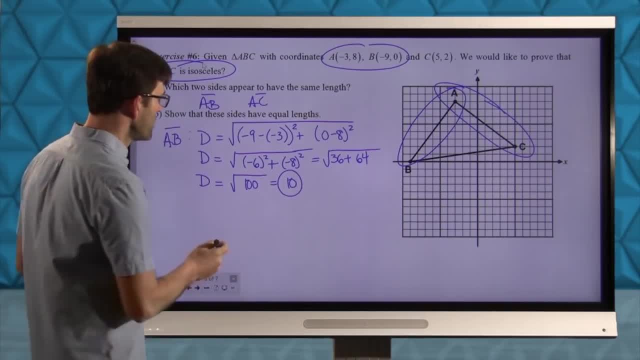 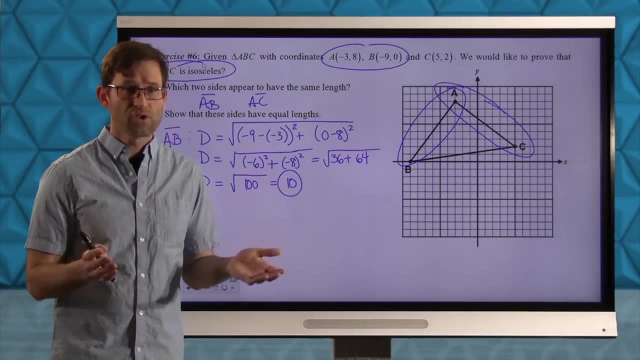 All right, Hopefully you can tell that's a 10.. Sorry, Anyway. Now, in order to prove that this thing's isosceles, we have to show it's got two sides, at least two sides that have equal length. 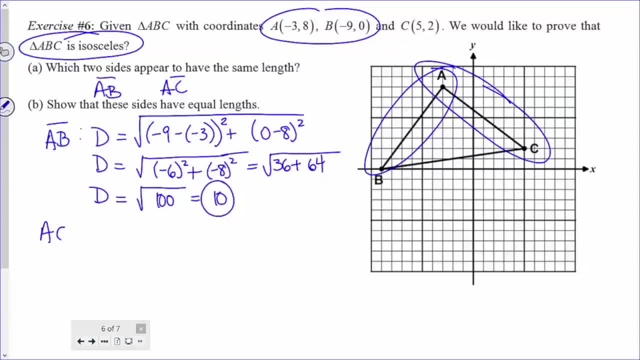 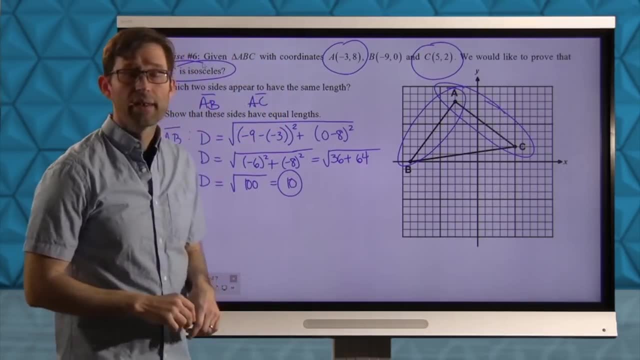 Now we have to go on and do the same thing for AC. So go ahead and work through the distance formula on AC right using these two points, And hopefully it will also be 10.. Now, by the way, if you're wondering to yourself, 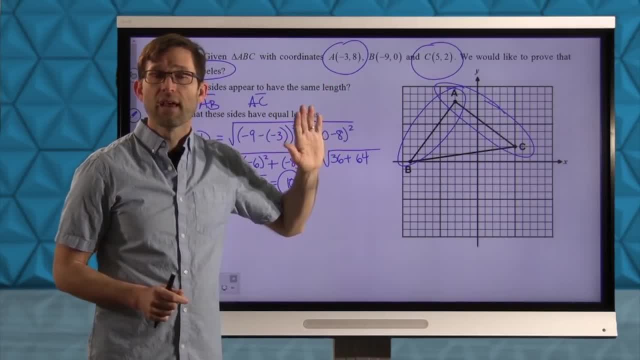 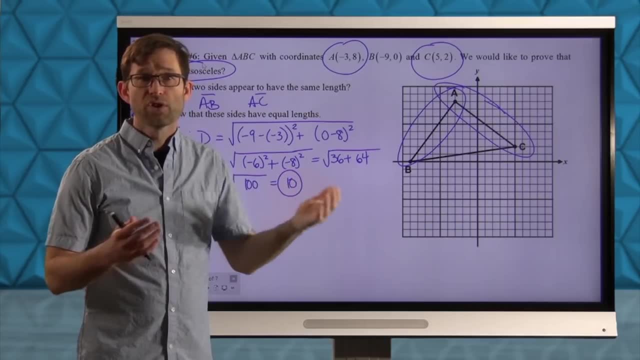 what do I use as x1, y1, and x2, y2,? the answer is: it doesn't make any difference. It can't make any difference, All right, But whichever way, whichever order you want to do it in, will work out just fine. 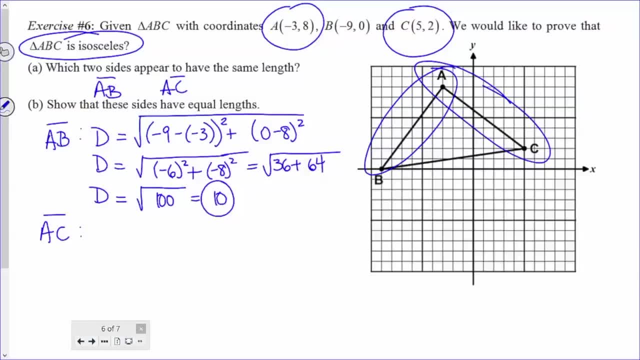 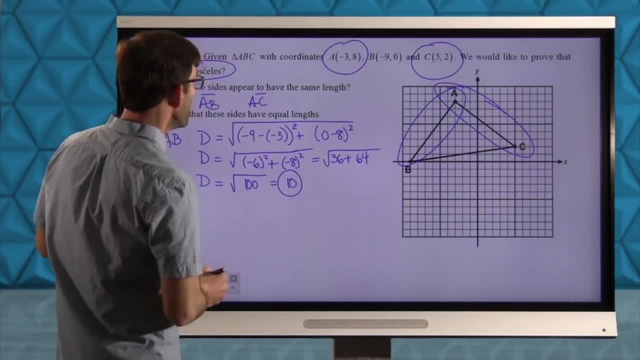 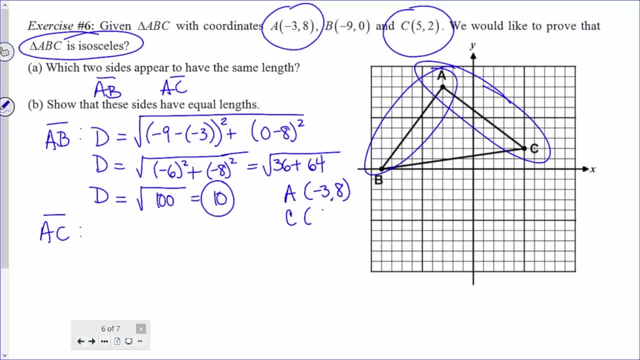 So take a few minutes and try to find the length of AC. All right, Let's go through it. Let me just write them down here, so I'll kind of have them, because I think I'm going to have to kind of move my board up a little bit. 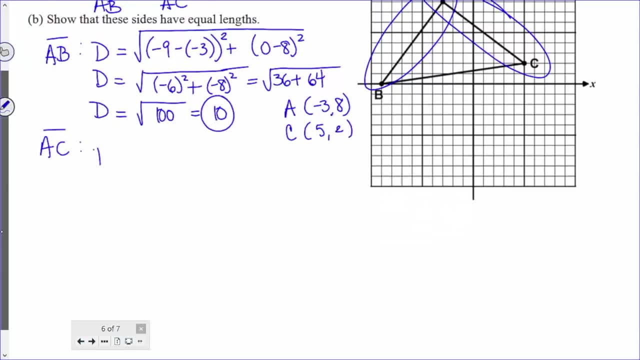 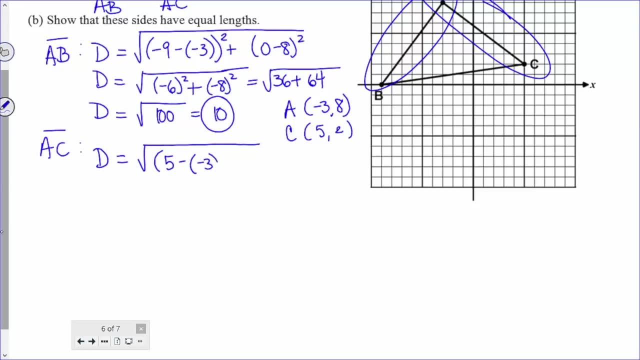 I just need those two points bring this up a bit. So the distance or the length of AC is going to be 5 minus negative 3, I think I'll go in that order: plus 2 minus 8, right, 5 minus negative 3 is positive 8.. 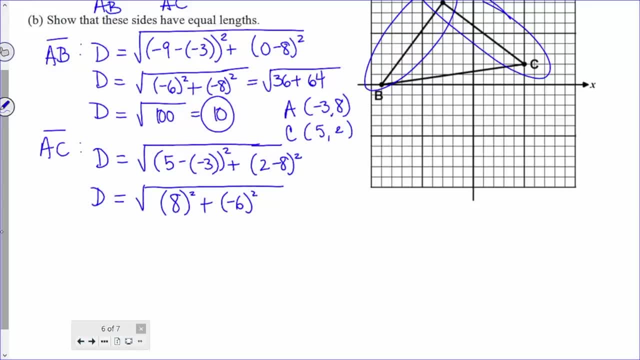 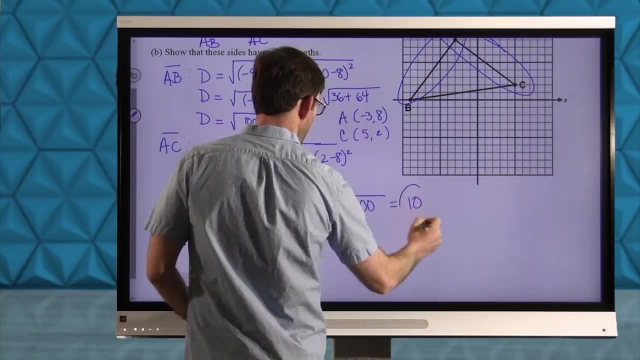 2 minus 8 is negative 6.. 8 squared will be 64.. Negative 6 squared will be 36.. Take the square root. I get a square root of 100 and 10.. And that's it Right. 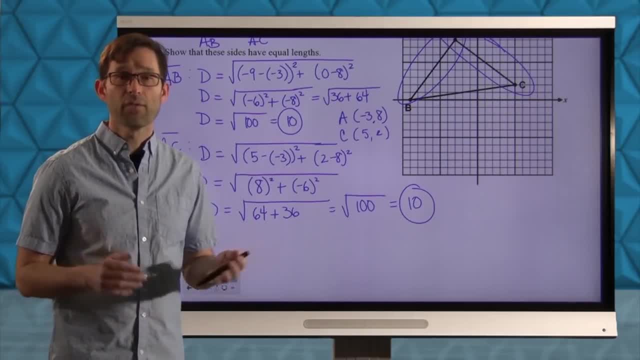 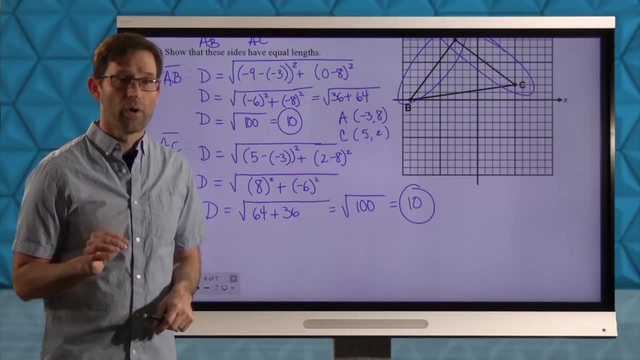 Those two side lengths must have equal length and therefore triangle ABC must be isosceles. And this kind of starts to get a little tricky. It starts to get into where we're going to eventually go with all of this, which is being able to use things like the distance formula. 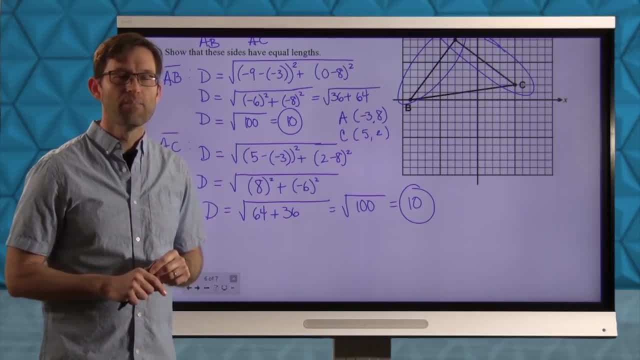 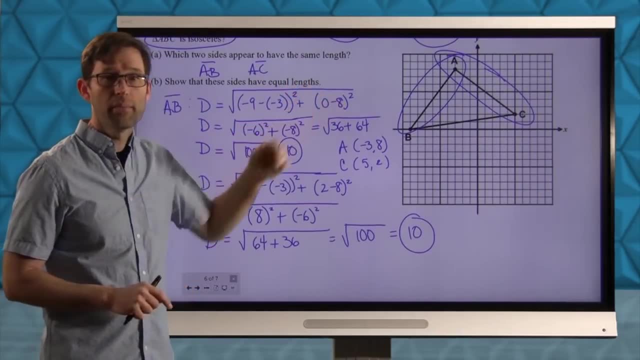 and the slope formula, and one more that we'll see in the next lesson, in order to prove things about geometric figures that happen to be in the coordinate plane, like triangle, ABC. All right, Take a little moment, if you have to, to write out that work. 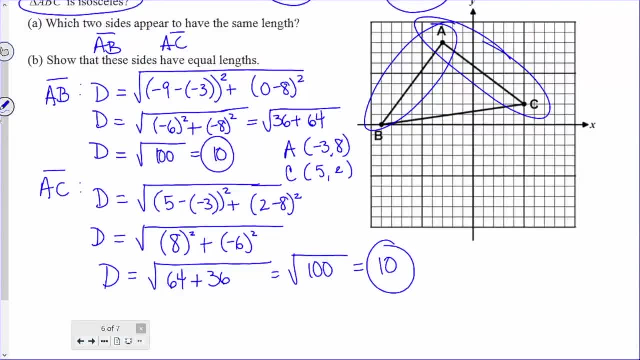 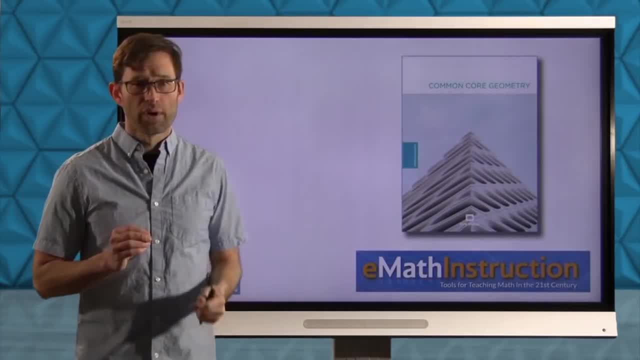 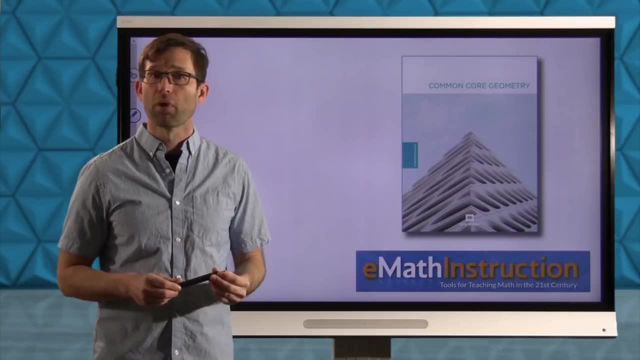 and then we'll wrap it up. Let's do it So. today we saw one of the major formulas of coordinate geometry, the distance formula. We even derived it And specifically it came from the fact that two points that are plotted in a coordinate plane along a slanted line. 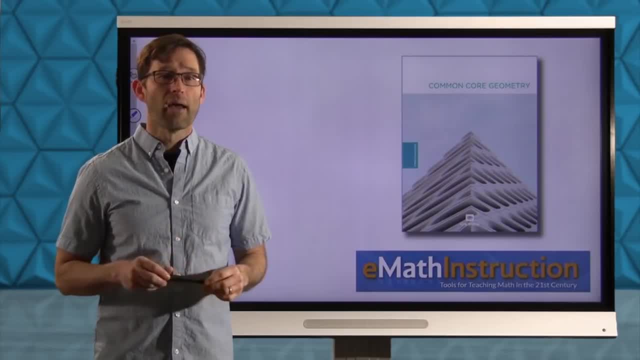 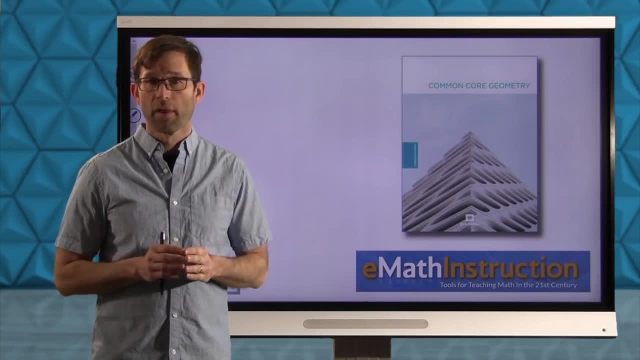 the segment that connects them can always be thought of as the hypotenuse of a right triangle. Using, then, the Pythagorean theorem, we were able to derive the distance formula that essentially said: look, find the distance between the x coordinates by subtracting. 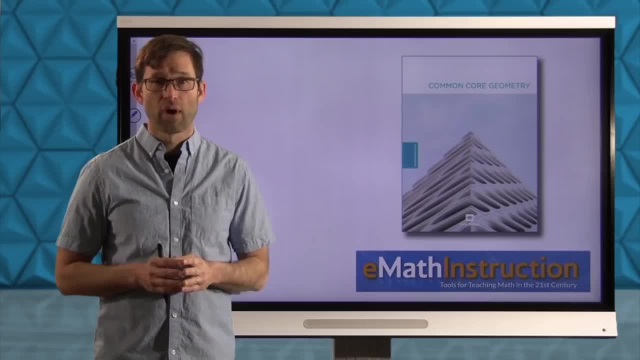 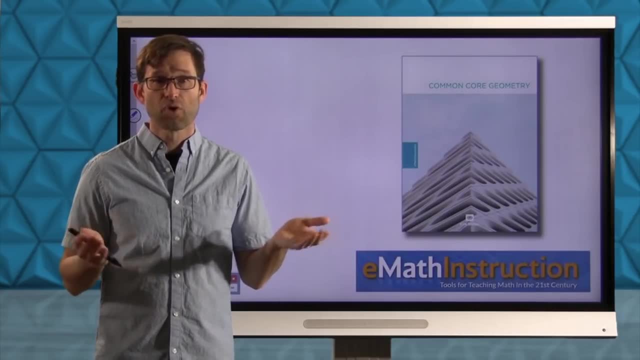 find the distance between the y coordinates by subtracting square those results, add them together and take the square root. That's the distance formula: Subtract, subtract, square, square, add together, take the square root. We're going to be doing that so much in this course.